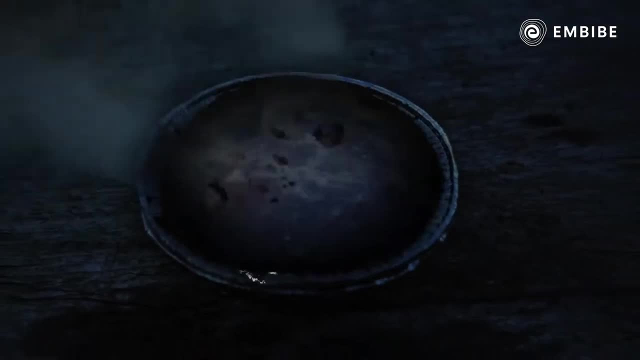 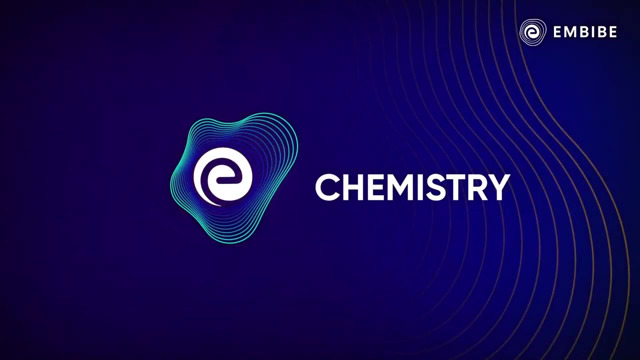 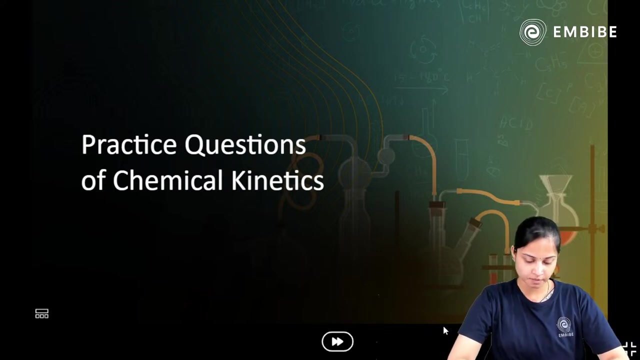 Hello everyone, a very good morning to each and every student present over here. It's me, your Raki ma'am, the chemistry mentor in front of you, And what we are actually going to talk about is today is the practice questions for chemical kinetics. 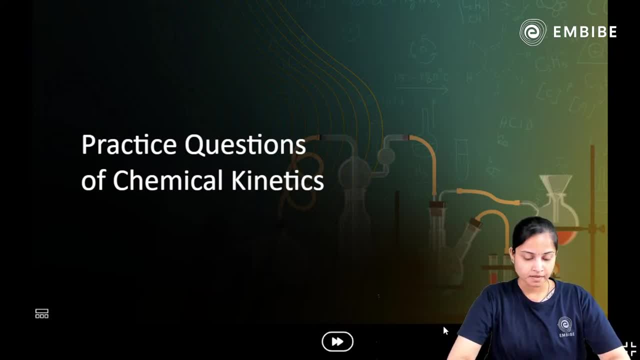 Hope that all of you have actually subscribed to the channel and I just request you people to please share this particular session as much as possible so that most of you can join this session on time. I know I am a bit of a delay. I mean to say I am going a bit of a delay today, So literally sorry for that particular thing. 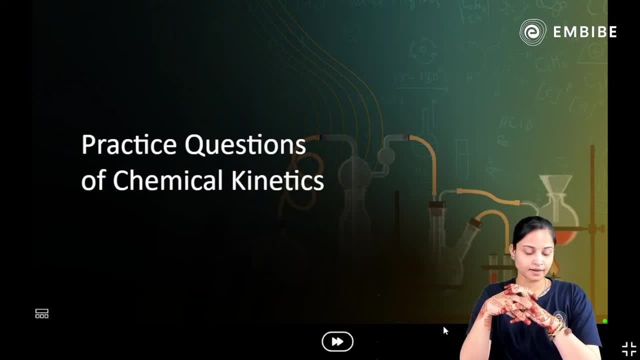 So, people, today what we are actually going to talk about is the practice questions for chemical kinetics. Yesterday we did a top 20 PYQs for chemical kinetics, Not top 20, I think only 10 to 11 questions we did for chemical kinetics. 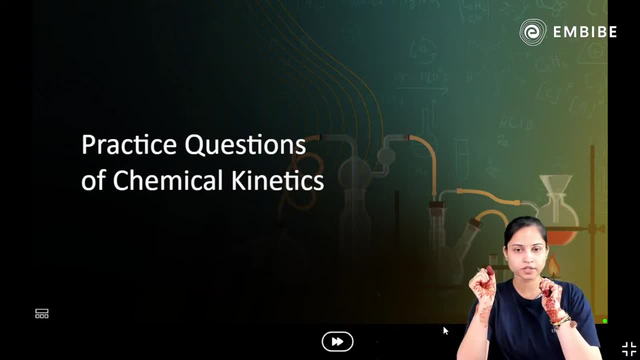 So today we will be practicing the good questions, good number of questions for chemical kinetics. I need your support. I need that you people should actually talk to me while we are actually solving the questions. The interaction is actually absolutely very important from your side. 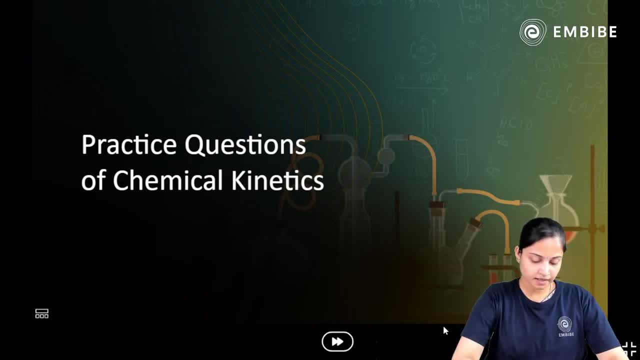 That's the main thing I literally want to talk about. Let's actually move ahead and talk about today's session. Well, I think all of you are in the bit of Actually, absolutely what. I just believe that all of you are in the best of your spirits and in the good health. 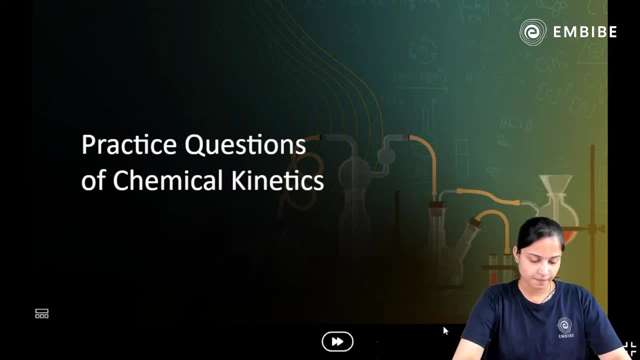 Hope everything is fine at your end, Isn't it? Yes, Okay, okay, okay. So let's move ahead and talk about the same. Here we are on to the point. So let's move ahead and let me talk about the things. 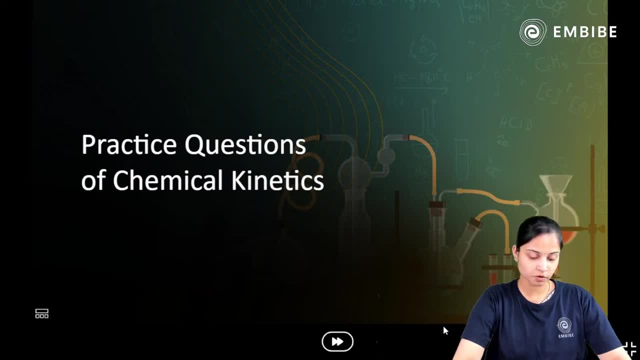 Fine. So people just say me: hello ma'am, hi ma'am, and just let me know if I am audible and visible to you people or not, Because each and everything should be on to the track. Yes, Yes, ma'am, absolutely. 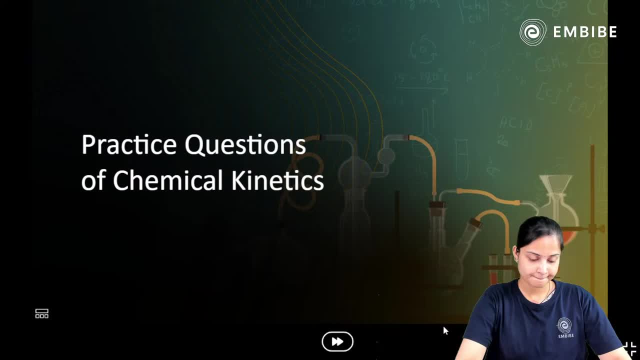 You are absolutely right, Okay, okay, Give me a few seconds so that I can just go ahead and talk about the same. Okay, and let me present you the questioners. Fine, just give me two minutes. Not two minutes, only seconds. 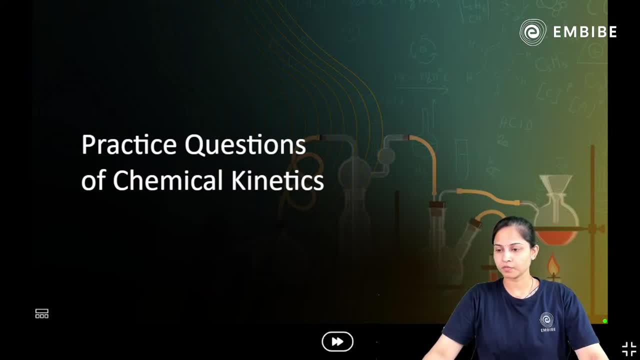 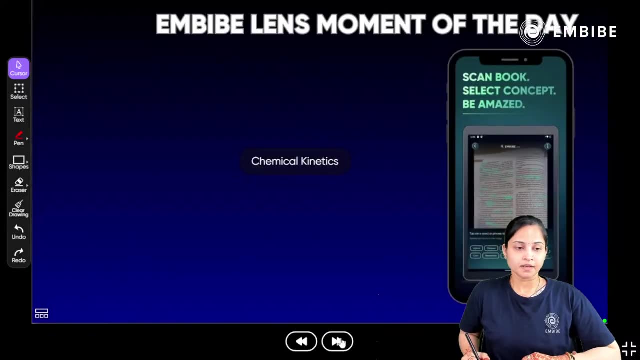 Yeah, here we are ready with the questions. also, I have imported the questions, So the thing, what you have to do is to tell me the right answer to the question. So, people, since NEET exam is very close to you, so you people need to do what. 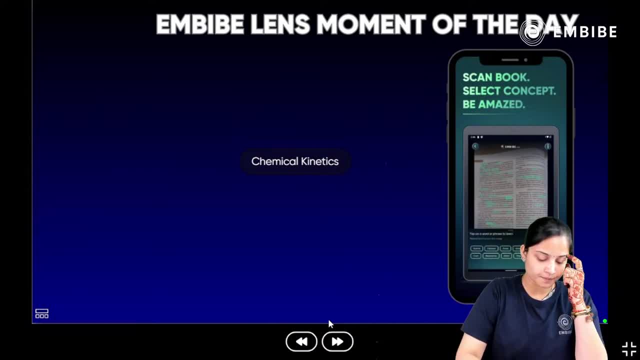 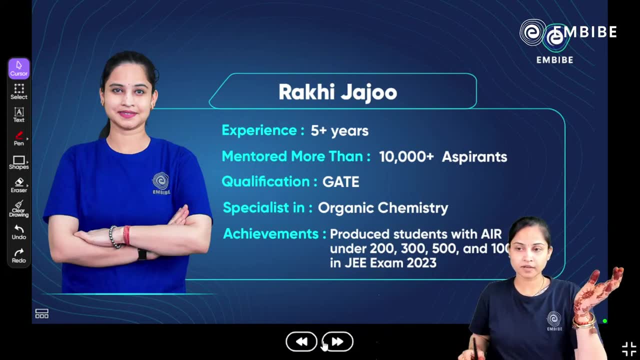 You need to work hard, you need to strive more. You have to give your 100% for the NEET examination. Let's move ahead and talk about this. This is all about your Aakhi ma'am, the chemistry mentor, in front of you. 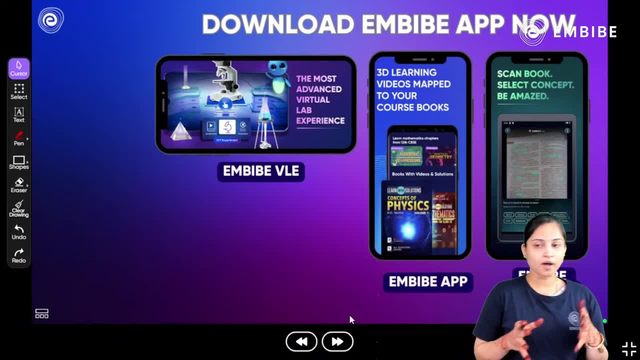 Talking about the MBIB app people. what do you Now have with you is the 7 days free trial. okay, You have 7 days free trial with you, so I just request you guys to please go ahead with these things. 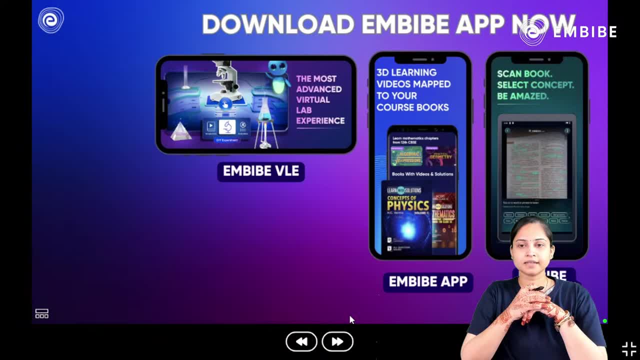 Reason being simple. I would like to say this to you all, and that is the thing that these three apps are: the mind-blowing apps, the wonderful apps you have ever seen. If I talk about, I just talk about the MBIB virtual lab experience app. so this is the app wherein you can perform the experiments the way you perform in your laboratory. 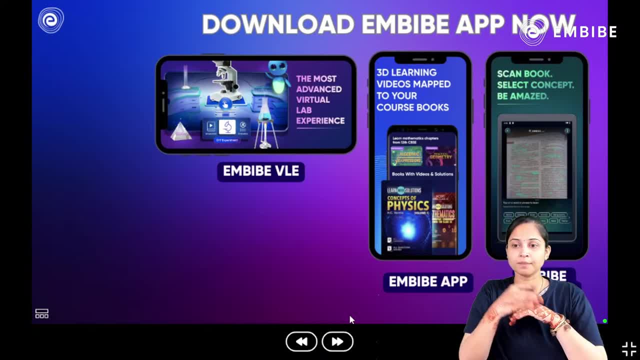 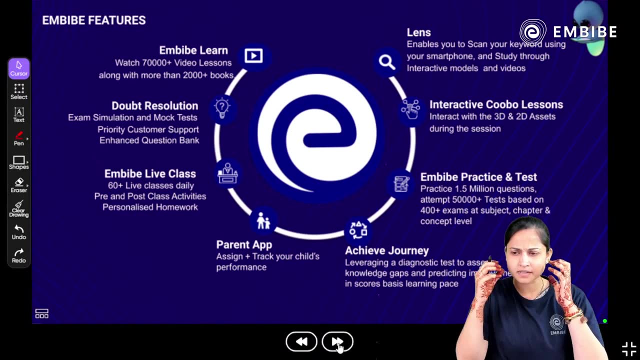 Okay, You can perform over here virtually Talking about the MBIB students app, and this MBIB students app contains these many features. basically, And these features are in itself the good features, the good number of features, I mean to say the features which is going to enhance your preparation journey for your examination. 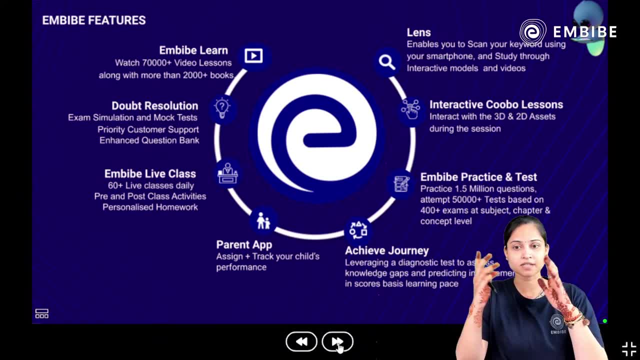 Hi Tapas. So MBIB Learn, Doubt Resolution, Life Classes, Parent App, Achieve Journey, MBIB Practice and Test, Interactive Google Lessons and the Lens- These are the mind-blowing features, So if you have any problem, you can perform over here virtually. 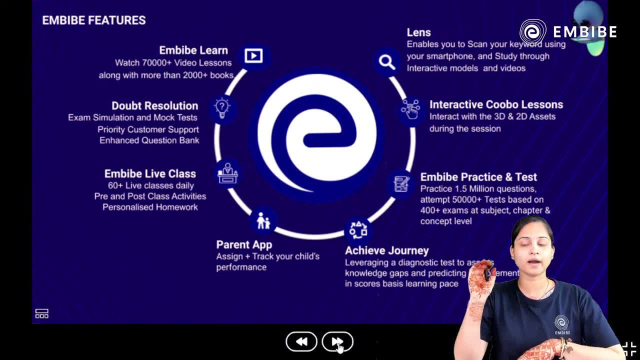 So if you have any problem in these particular features, I request you people to just go and watch out the Ankana ma'am videos. She has uploaded the videos individually on each and every feature of the MBIB So you can just have a look over there if you have any problem regarding them. 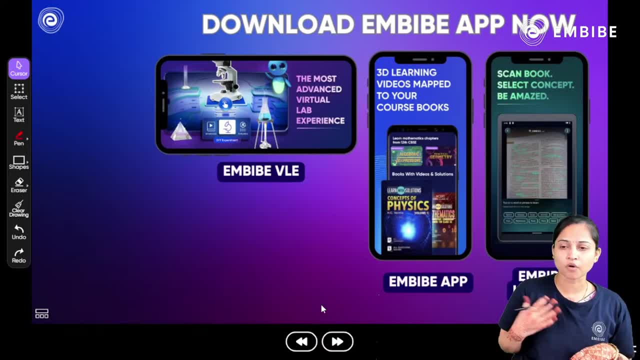 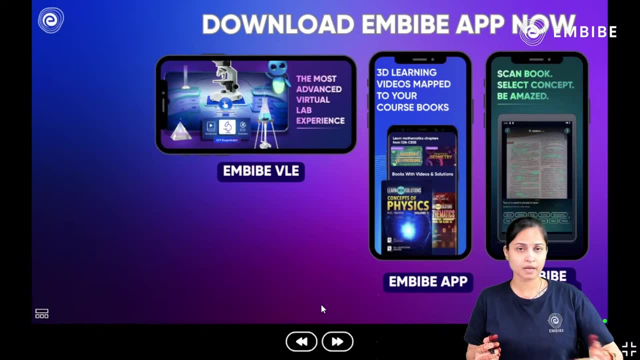 But if you will explore all the features, you will find that these all features are, in a way, somewhere or the other, going to help you out in your preparation journey, Whether it be NEET exam, whether it be JEE exam or whether it be board examination. 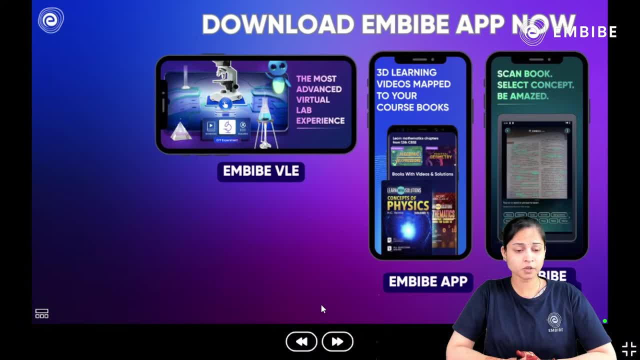 Talking about the MBIB Lens app People, let me tell you about the MBIB Lens app. So if you are reading a book- obviously if you are reading Physics, Chemistry, Mathematics, Biology, any book- and you feel there is some problem, you are not able to understand anything. 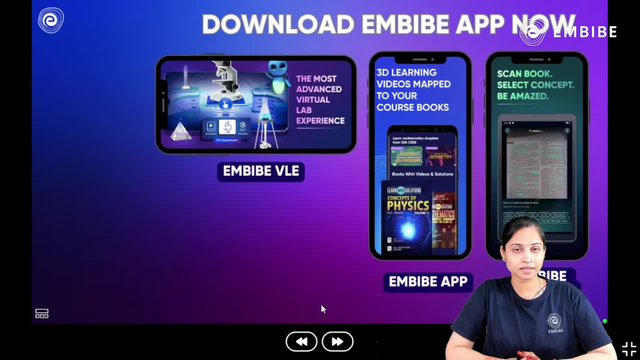 You can do one thing: You can just take the snip of that particular text or the content, upload it over here on the MBIB Lens and within fraction of seconds- not fraction of seconds, I shouldn't lie- It's a matter of 10 to 15 seconds. 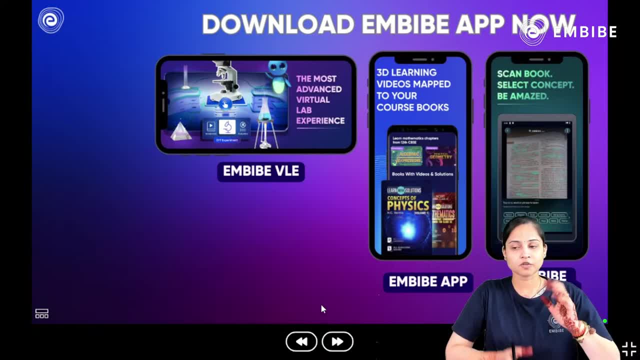 You are going to get the simpler version of that particular thing. So if you are getting the simpler version enough to understand that particular content or the text along with it, you are going to get a surprise- that is, the 3D view model- along with that particular simpler version of the text. 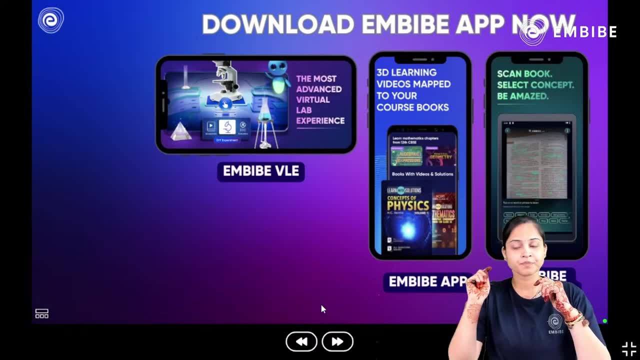 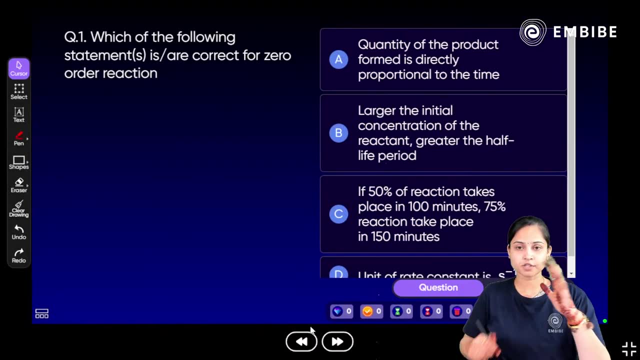 You are going to snip over here, You are going to upload it over here, So just trust me, each and everything is going to be fine over here. Let's actually move ahead and talk about the very first question which is in front of you. 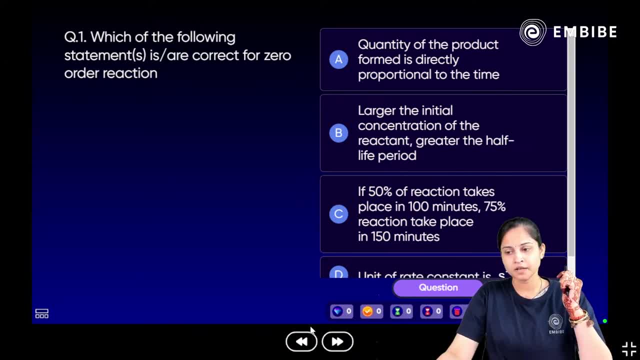 which of the following statement is, or are, correct for the zero order reaction. So this is what you need to actually talk about. Let's move ahead and talk about the same. What do you have to say? What do you have to say about this particular thing? 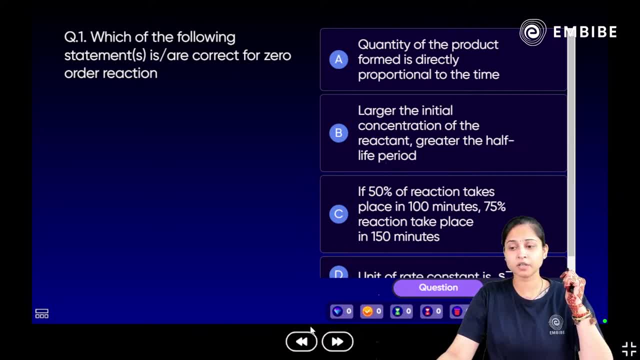 Which of the following statement is, or are, correct for zero order reaction? And let me tell you one particular thing: that most of the questions you are going to get into your NEET examination belongs to zero order as well as from the first order. So ya tapas the very first question onto the screen for you people. 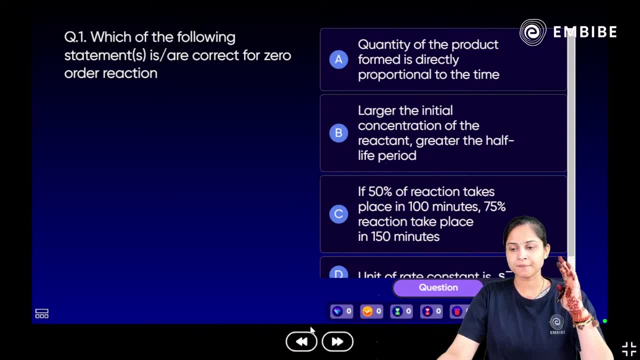 So let me know the right answer to the question over here. Take care So which of the following statement or statements is, or are, correct for zero order reaction? Tell me. The statement 1 says quantity of the product formed is directly proportional to the time. 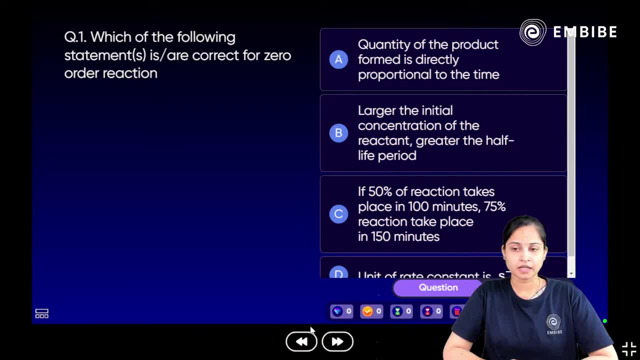 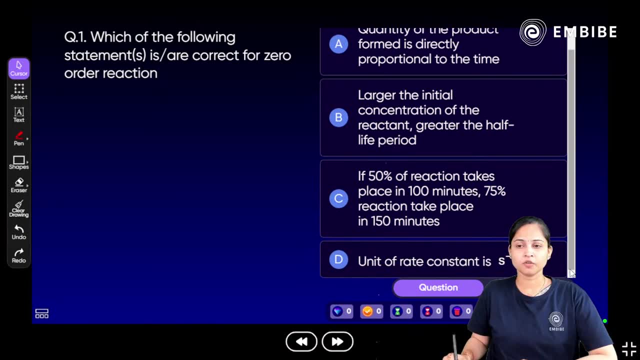 Larger the initial concentration of the reactant, greater the half-life period. If 50% of the reaction takes place in 100 minutes, then 75% of the reaction takes place in 150 minutes. Unit of rate constant is second inverse. 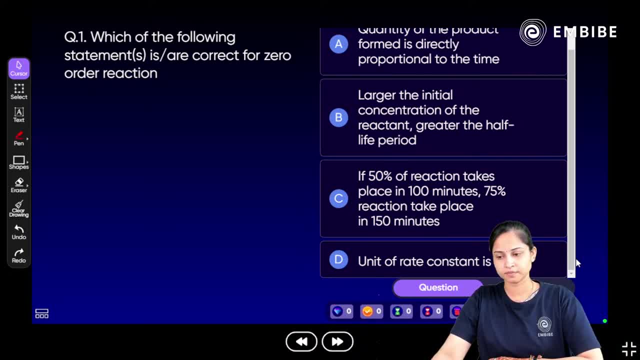 Let me know the right answer to the question. What do you all have to say about this particular question? I'll explain you each and everything, Everything over here, need not to worry. Just let me know the right answers to the question over here. 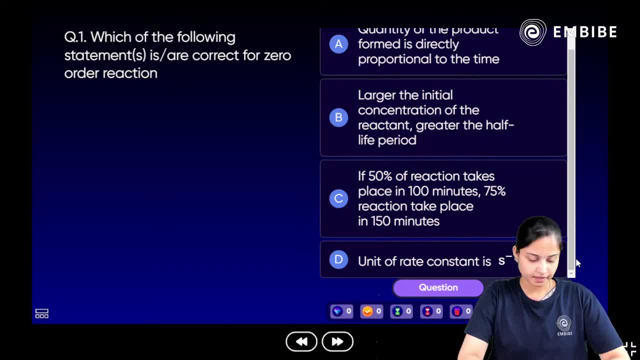 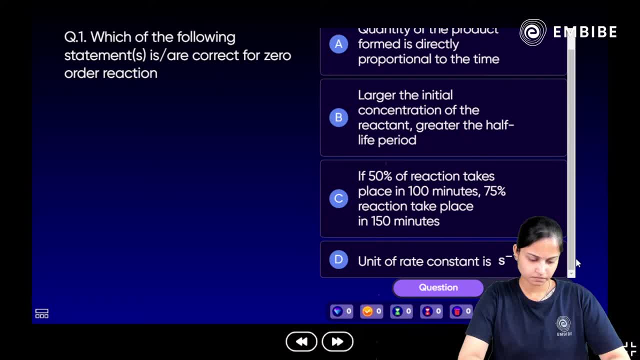 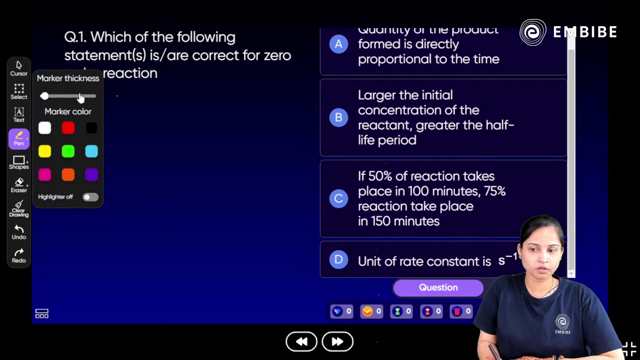 Thank you. So I think you haven't answered me anything over here, So let me actually go over the things. So if I want to explain the first statement, then I'll do it Here. do you know what we know for zero order? 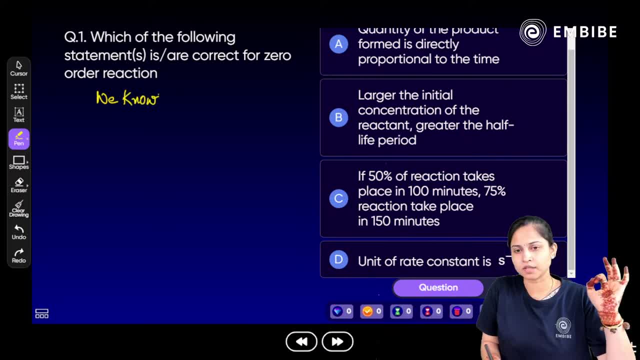 See, we know that for zero order. I'll explain every question very well. We know for zero order. We know for zero order reaction. What we know for zero order reaction: Yes, Like our product is being made from A, Is it clear? 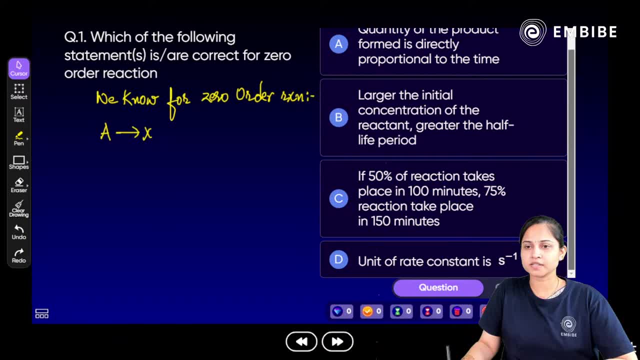 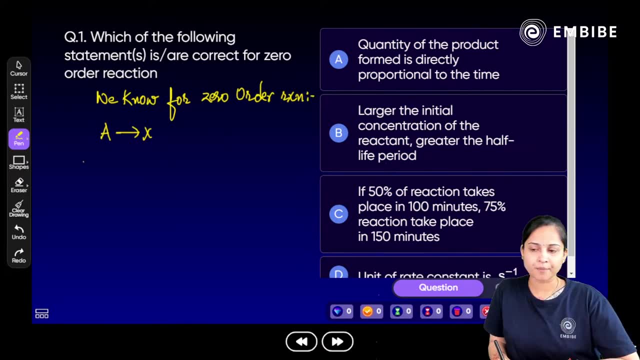 Yes, So I'm explaining the first statement to you, Wherein they are actually saying us: the quantity of the product formed. Quantity of the product formed is directly proportional to the time. So you know this much that if I talk about rate Rate, R is equals to K A raised to power zero. 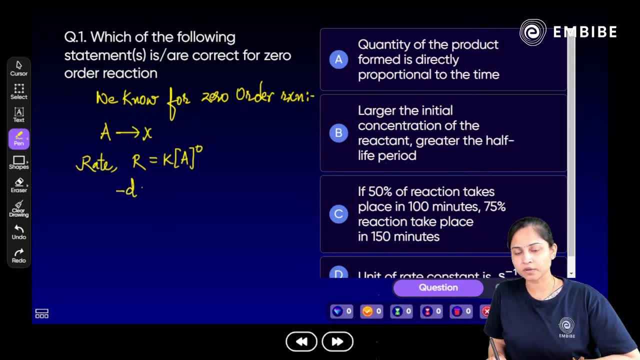 That's for zero order reaction. So what can I write over here? Rate of disappearance of A that is minus dA by dt is equals to K. A raised to power zero, Isn't the thing clear? And something raised to power zero is equals to one. 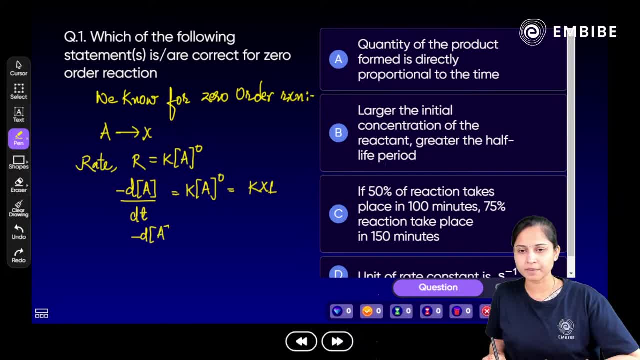 So K into one, So minus dA. Now it becomes equals to K, dA, Dt. What has become? It has become K, dT. So what over here we are actually going to talk about That? the product so formed is directly proportional to time t. 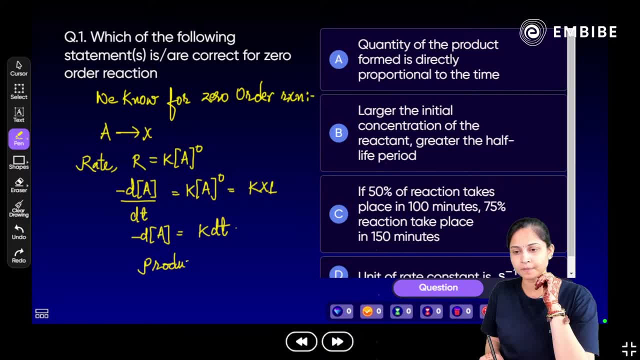 The product so formed. Product Formed Is directly proportional to time, t Am I right? Am I making things clear to you? Yes, So the quantity of the product formed is directly proportional to time. Yes, A is the right answer. 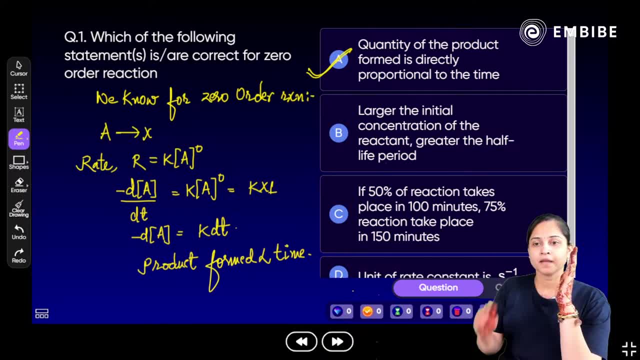 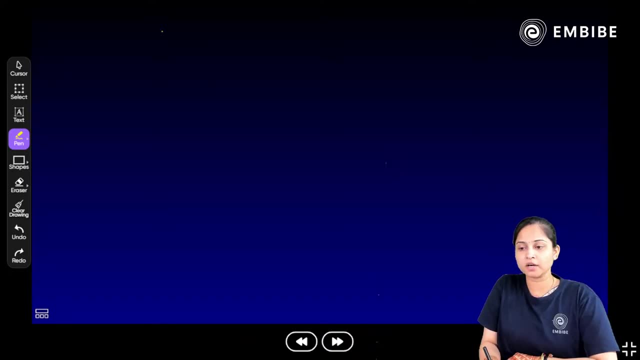 The second question, which they are actually absolutely statement. they are asking us: Larger the initial concentration of the reactant, greater the half-life period. Larger the initial concentration of the reactant, greater the half-life period they are actually talking about. So over here what I literally want to talk about for the second statement: 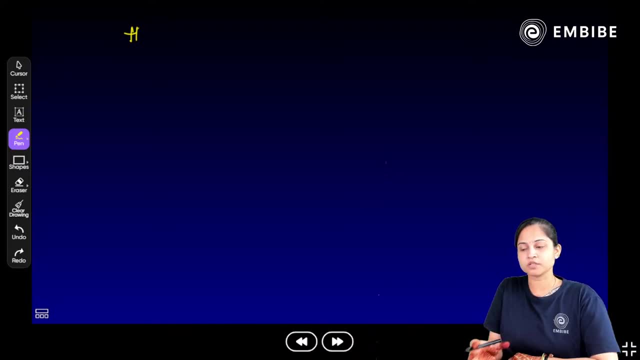 K. half-life is the time at which the concentration becomes half of its initial concentration. Half-life is the time at which the concentration becomes half of its initial concentration. So when I just talk about the Half-life time, Okay, That means t is equals to t half. we are going to talk about 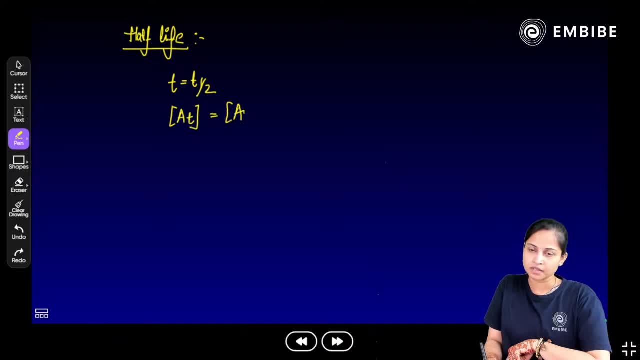 Herein we can say the concentration, which was 80. now it becomes half of the initial concentration. And what we know for zero-order reaction? We know for zero-order reaction that 80 is equals to a naught minus kt. The integrated rate law equation. 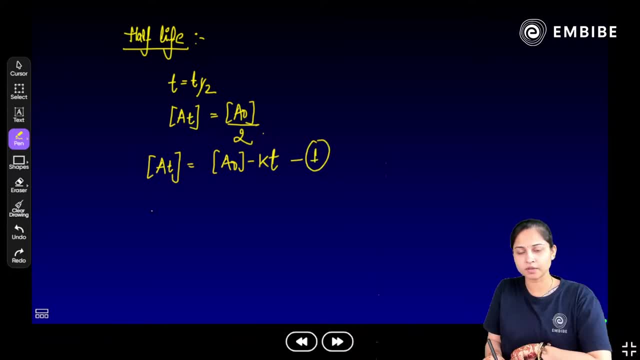 This is our equation number 1. Substituting the value of 80 over here, So it's basically a naught by 2. Minus a naught and it will be minus kt of half. basically, Tell me, Did you understand this? 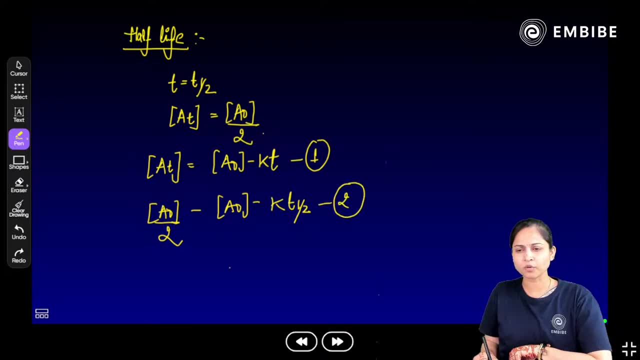 Is this our equation number 2?? Yes, So from here what we actually got. What did we learn from here? We learned from here that t half is equals to a naught by twice of k, Which what it does mean. It means that t half is directly proportional to a naught. 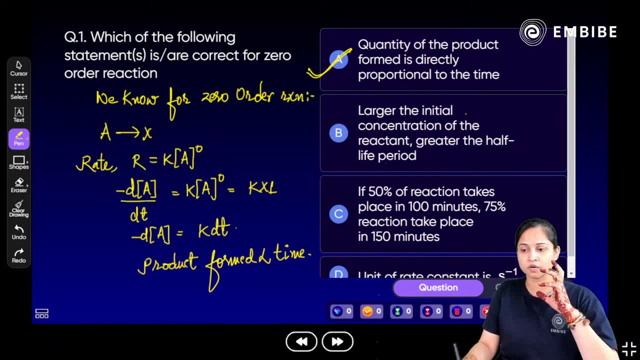 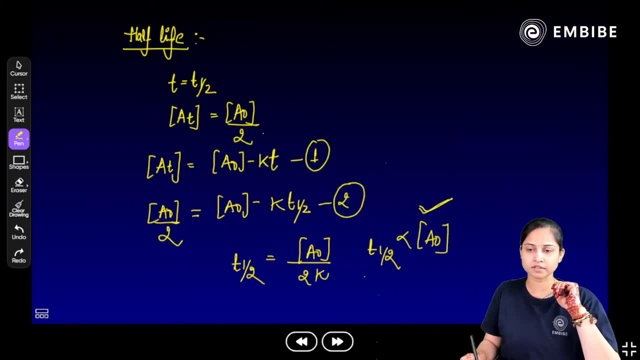 And this is what they were actually asking us. Larger the initial concentration of the reactant, greater the half-life period. So larger the initial concentration of the reactant, greater the half-life period. That is absolutely the right one. Okay, So option B is also the correct statement. 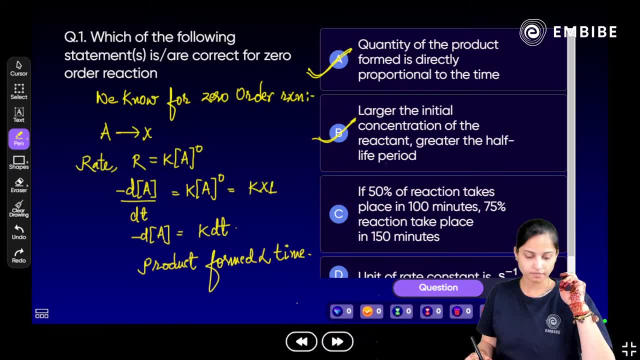 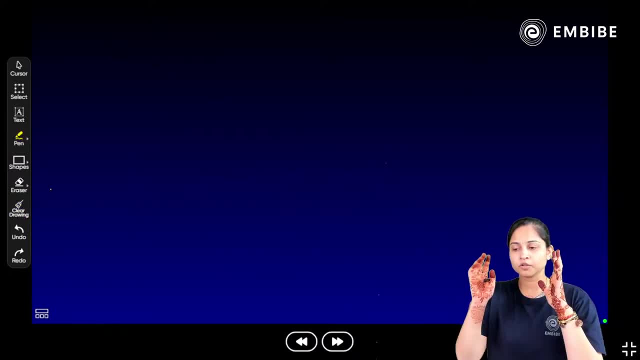 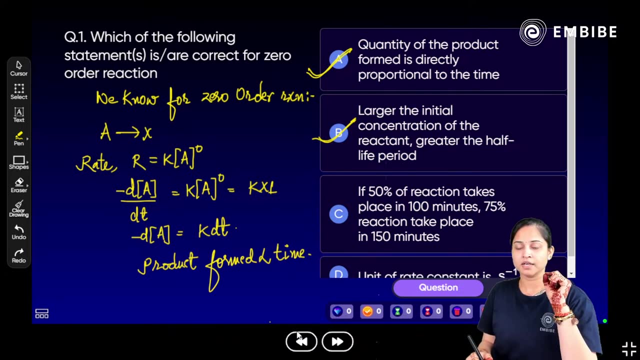 Now let's actually buy for option number C. Let's look out for option number C, what we actually want to talk about. If I talk about option number C, So using the integrated law equation for zero-order, You see here The reaction takes place in 100 minutes. 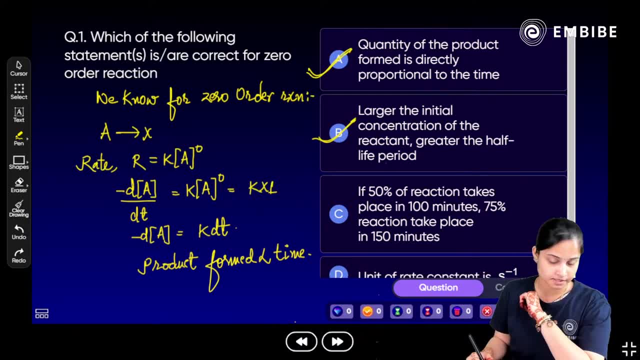 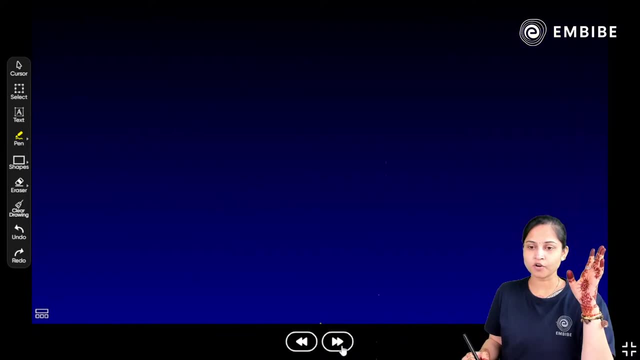 75% reaction takes place in 150 minutes. Yes, Tell me, what will you say for this? What do you have to say about this particular thing? So here we need to buy something for option number C also. So for option number C, if I just say using integrated, 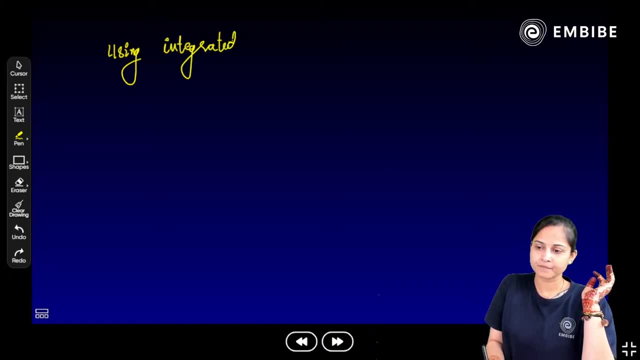 Using integrated law equation, Using integrated law equation for zero-order, for zero-order, basically. So, at 50% of reaction, at 50% of reaction, What I literally want to talk about over here, at 50% of the reaction, I want to talk about the. a naught minus a naught by 2 is equals to K into 100. 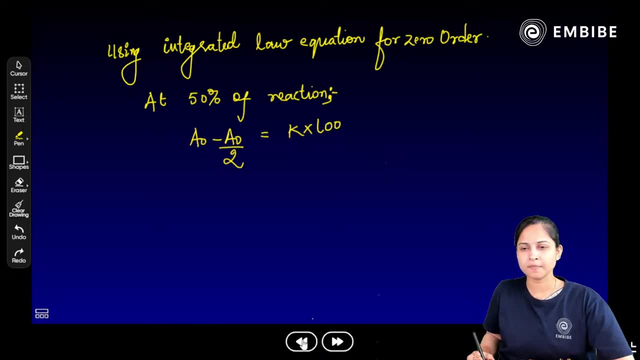 Because we have been told that when 50% of the reaction gets completed in 100 minutes, So at 50% of the reaction, a naught minus a naught minus a naught by 2, which is equals to K into 100.. 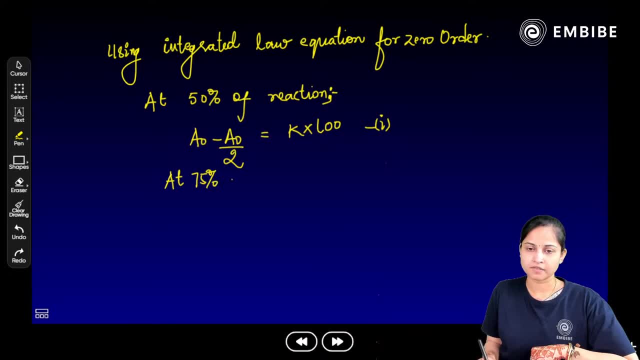 At 75% of reaction, At 75% of reaction basically. So it is a naught minus a naught by 4.. Which is then equals to K, into T, and this is the second equation, If I just divide 1 by 2, dividing 1 by 2.. 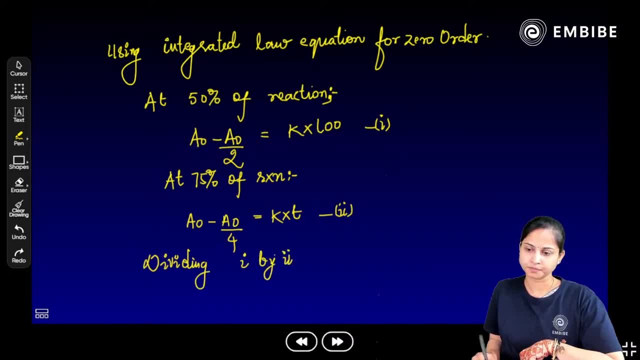 Dividing 1 by 2.. So if I do so, So it becomes a naught by 2 by 3, a naught by 4. Which is then equals to K into 100, by K into T. That's absolutely right. 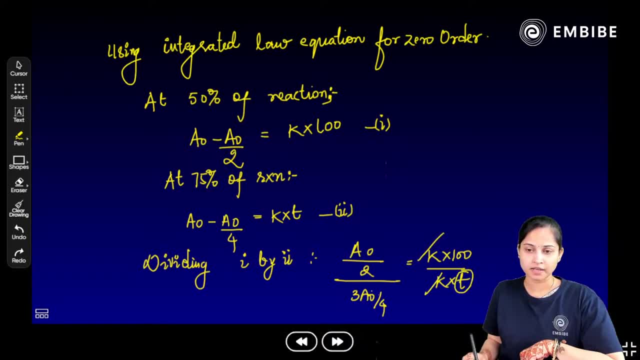 So we need to find out the value of T. K cancels out with K, A naught cancels out with a naught. basically, Yes, people, let me know. So from here, the value of T comes out to be equals to 100 into 3 by 2.. 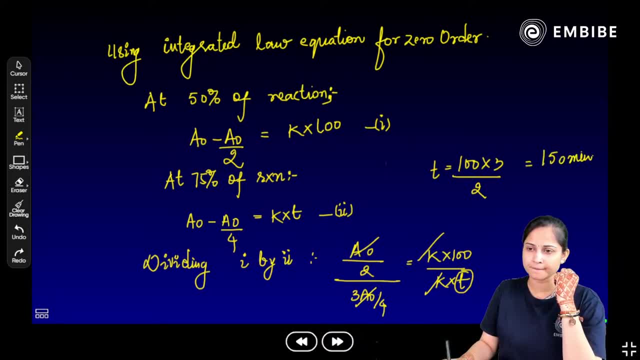 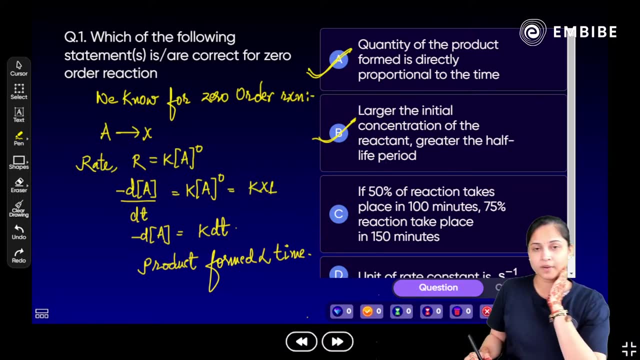 So it is equals to 150 minutes. Yes, for 75% of the reaction to be completed, 75% of the reaction to get completed, It requires 150 minutes over here. Yes, so option number C is also right. So we did 3 questions. 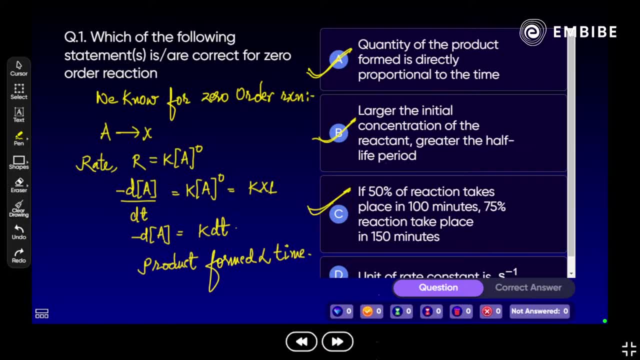 We did 3 questions in 1 question. We did 3 questions in 1 question. Yeah, people tell me We did 3 questions in 1 question over here, Am I right? Yes, So in a way, now our last statement. 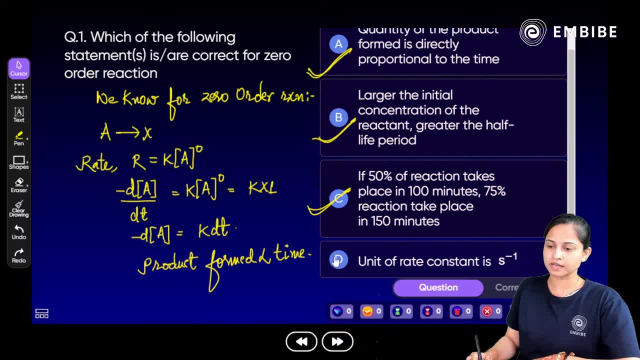 What is the last statement asking us? Unit of rate constant is second inverse. Do you really think so? unit of rate constant is second inverse. No, Unit of rate constant is not second inverse. Rather, if I just talk about unit of rate constant, 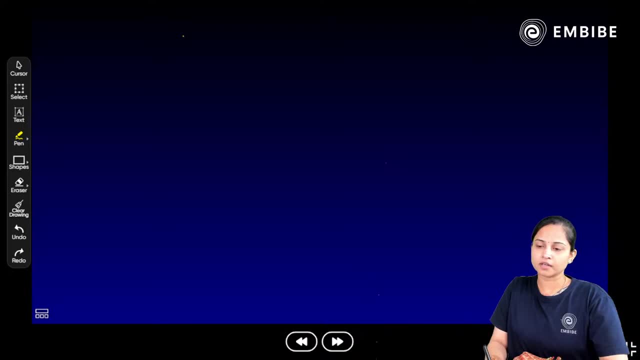 So, people, I want to clear one thing That we know that K is equals to a naught minus 80. By T. So unit for K, Unit of K for zero order, Unit of K for zero order reaction is mole liter inverse. second inverse: 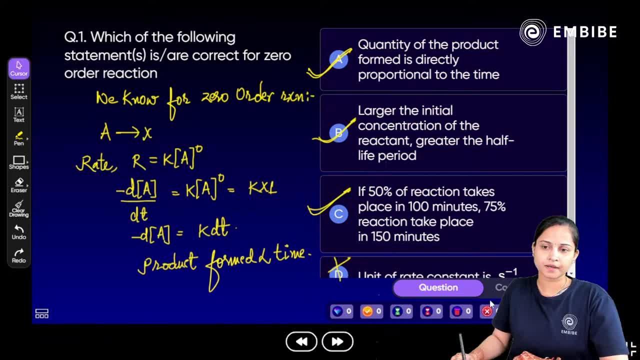 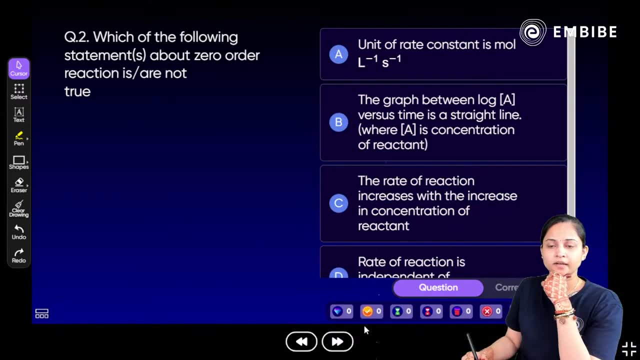 So only statement number A, B, C are the right statements. The correct answer to the question is this: Good morning, Aditya. Let's move on to the next question. Over here again we have C. We have done 3 questions. 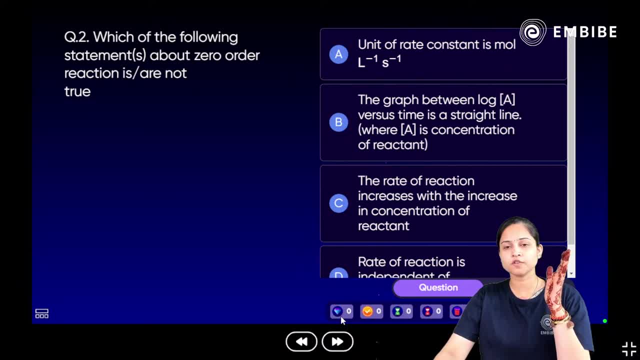 We have discussed 3 questions in a way. Now, which of the following statements about zero order reaction is or are not true? What have we been asked? Not true? So let's see what is not true for zero order. Unit of rate constant is moles per liter per second. 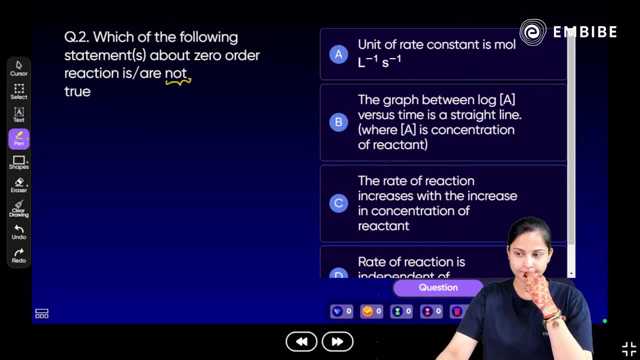 Unit of rate constant. tell me: Unit of rate constant is moles per liter per second. Unit of rate constant is moles per liter per second. Yes, this is the true statement We want to know, not true. Now the graph between log A versus time T. 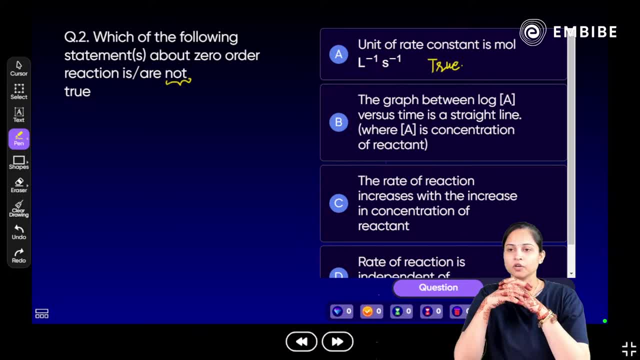 Yes, people, The graph between log A versus time is a straight line. Where A is concentration of reactant, Where A is concentration of reactant, Where A is concentration of reactant. Graph between log A versus time T. Graph between log A versus time T. 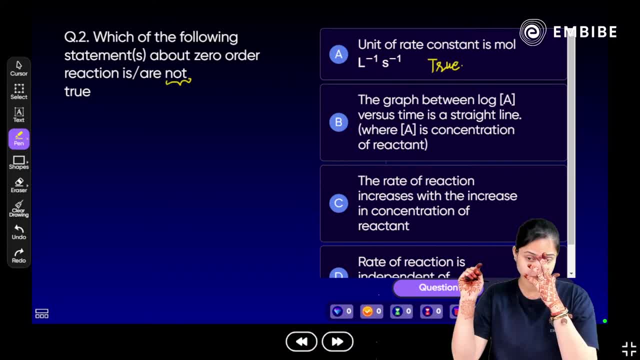 Tell me what you have to say. see here, I want to say one thing, and that is a thing if I just talk about for option. I will be talking about statement number 1. so if I am considering A to B reaction, ok, so rate law for 0: order reaction is given as: 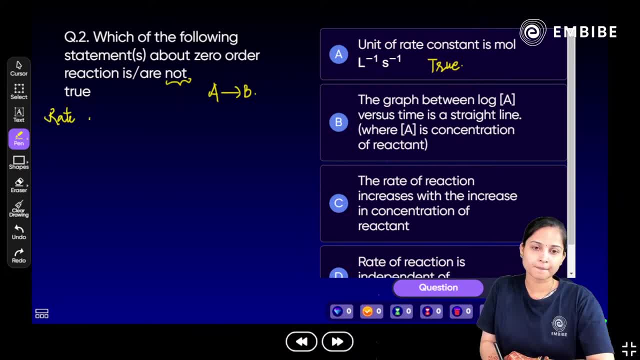 rate law for 0: order reaction. rate law for 0: order reaction. so rate R is equals to K. A raise to power: 0. fine, we know that. then minus DA by DT is equals to K. A raise to power 0. minus DA by DT is equals to K into 1. 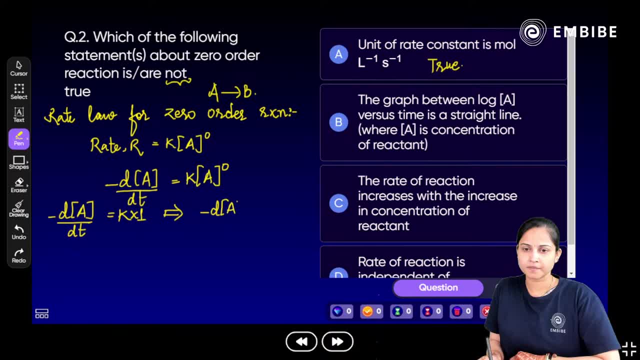 minus DA is equals to K DT. so if I just take the limits on both the sides now, it's A naught to A T and it is DA minus bar equals to K 0 to T DT. ok, so if I say when time is equals to 0, 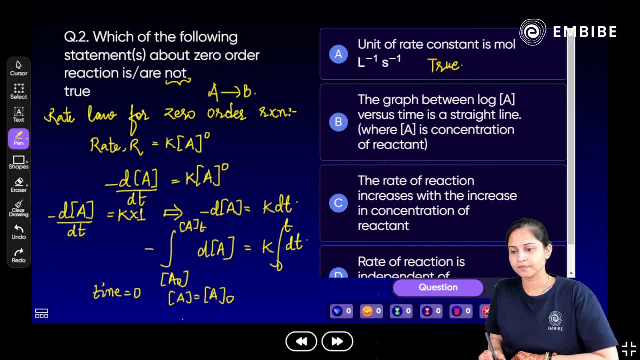 so our A will be equals to A naught, and when time is equals to T, so our A will be A T. you understand this? this is all what you know, people. that is the main thing. yes, so if I solve these limits, the thing which I am going to get is: 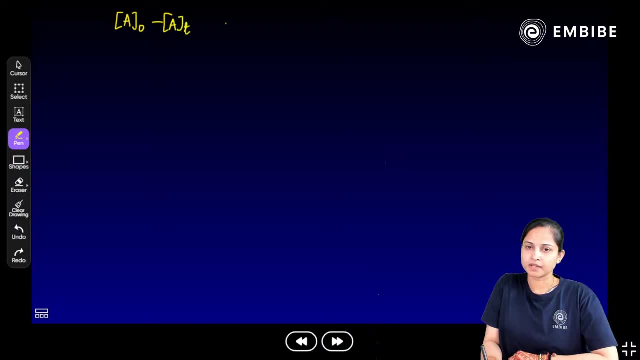 A naught minus A T is equals to K T. ok, wherein I will just say that A T is equals to A naught minus K T. what is this? this is equation 1. this is equation 1. what is A naught? initial concentration is of reactant A. 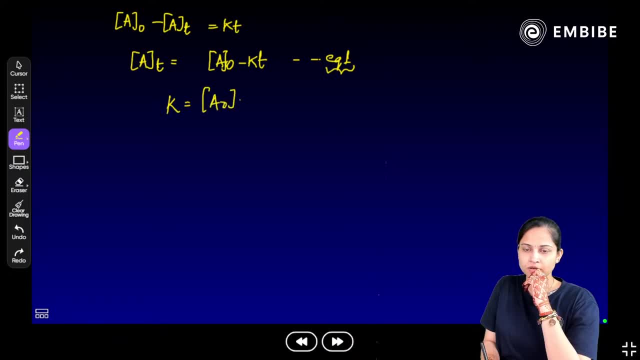 so from here, what is K? it is A naught minus A T by T. ok, is it clear here? ok, now let me tell you that in unit of zero order, I know that moles per liter per second. but if I take log, where is this equation? 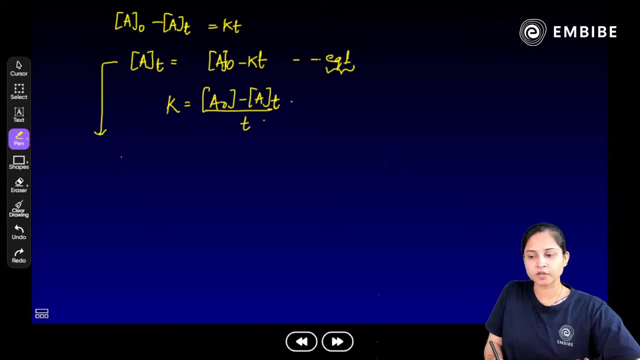 if I take log from both sides, taking log for equation number 1, so it is log of A. ok, it is equals to log of A naught minus K T. This is our second equation. Equation 2 is not in the form of which particular form you want. 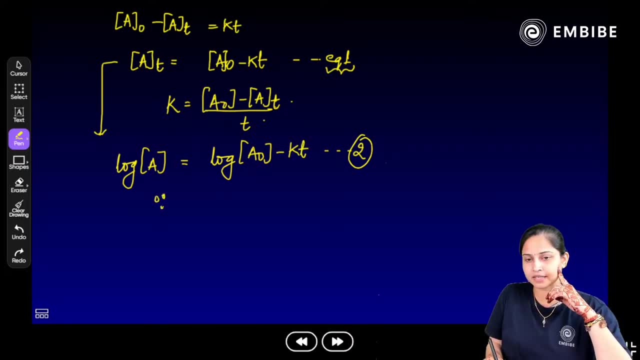 Yes, equation 2.. Here you can see that, since our equation 2 is not in the form of log, a is equal to mt plus c, So log a versus time t will not be a straight line. So this is our false statement. 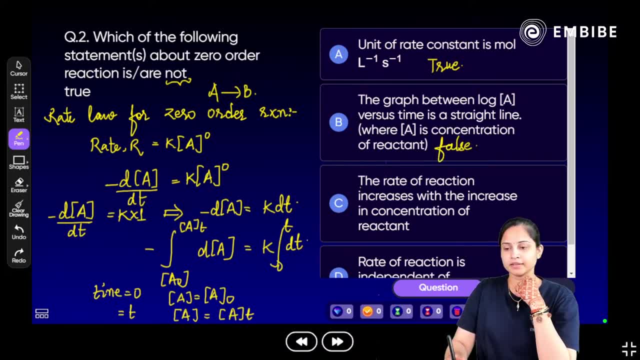 It will not be a straight line. basically, That is absolutely right. The graph between log a versus time t is not a straight line. That will not be a straight line, people. It will not be a straight line. Will it be a straight line? No, 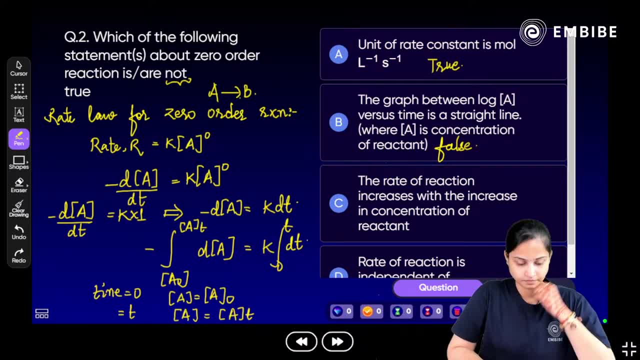 That won't be a straight line. Tell me That won't be a straight line, So false. Now the rate of reaction increases with increase in the concentration of reactant. I would like to tell you one thing Here. you would know one thing. 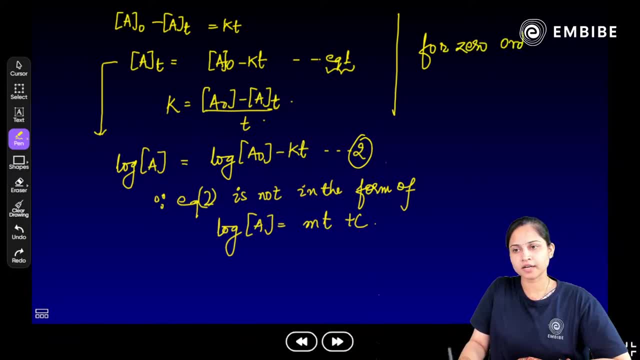 For zero order reaction. You all know what happens for zero order reaction. For zero order reaction, The rate which is there, Rate r, is equal to k, That is, it is the rate constant. Okay, Now, rate of zero order reaction. Whose rate is this? 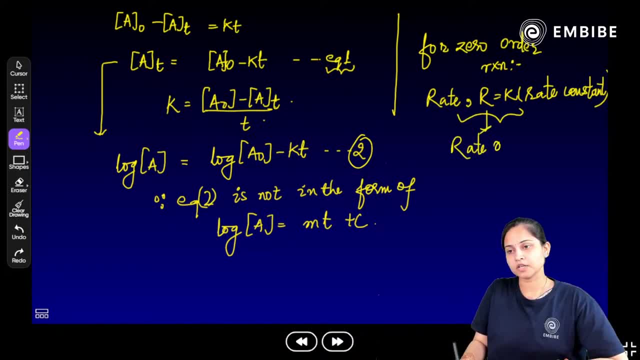 Rate of zero order reaction. Rate of zero order reaction. Okay, So rate is equal to k rate constant. So rate of zero order reaction, Rate of zero order reaction, is equal to rate constant of that reaction Which is independent of the concentration. 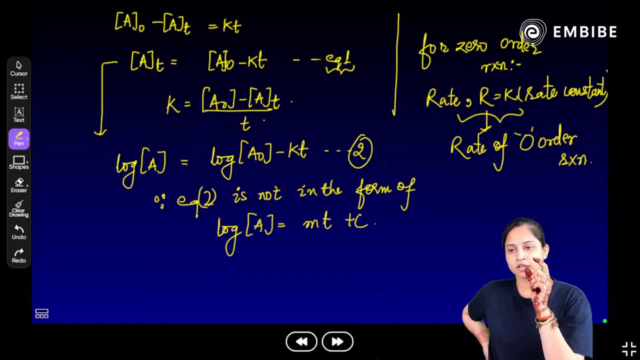 Hence, on increasing the concentration of the reactant, Rate of reaction does not increases. So if I make a plot Of rate versus concentration, If we plot the plot of rate versus concentration, So we are going to get this particular graph, We will get this graph. 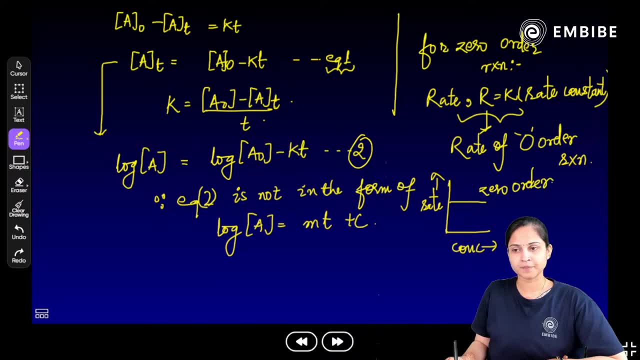 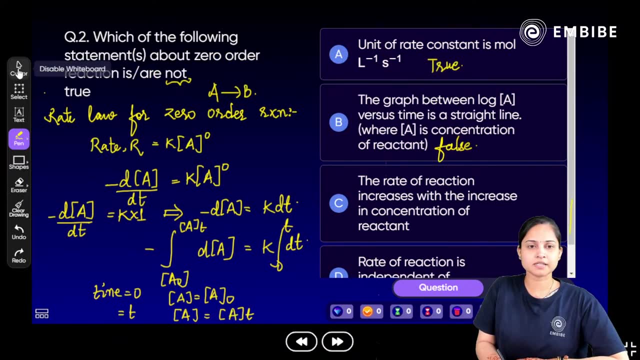 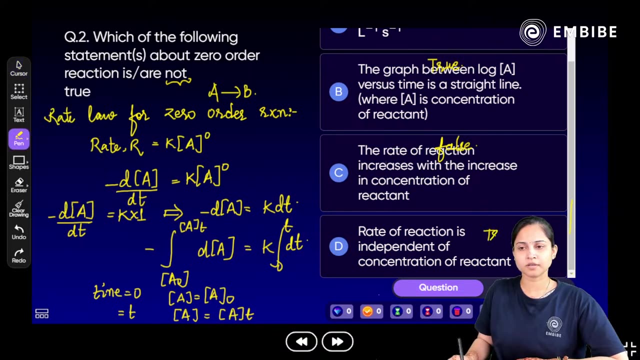 We have told you in respect of zero order. Okay, Is this clear? Okay, Talking about the last statement, What does this say about the last statement? Rate of reaction is independent of the concentration of the reactant. Yes, This is our true statement. 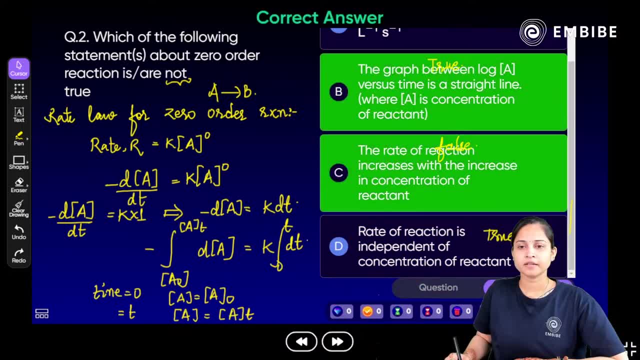 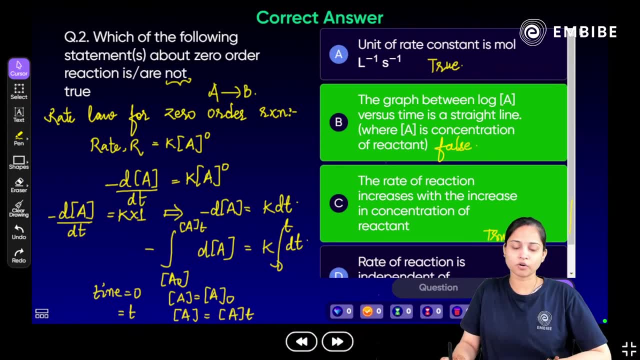 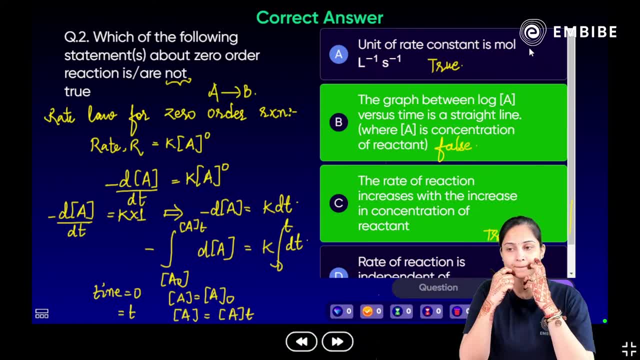 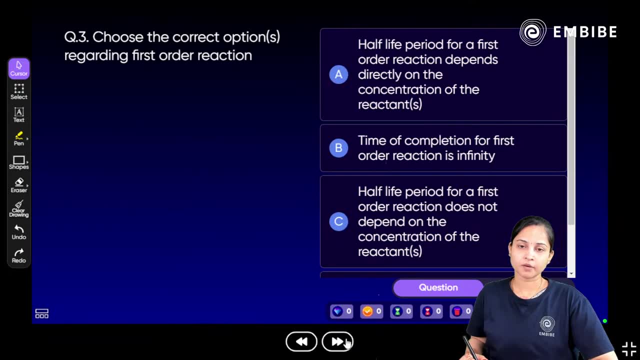 Shall we move ahead, Shall we move ahead. Just let me know, Let's move ahead and talk about the next question. Here we are on to the next question. Question after question is also a statement type of a question. Now you have to talk in respect of first order. 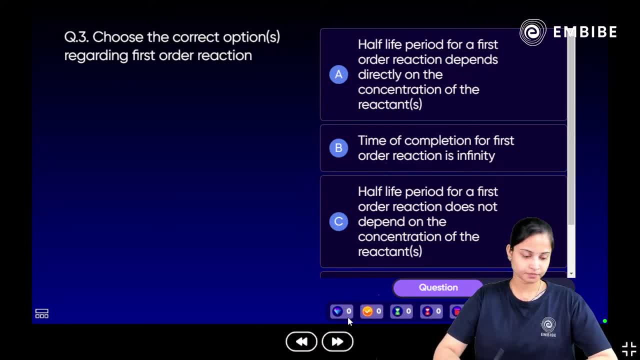 Choose the correct option or options regarding first order reaction. Okay, I am giving you the time. We have solved how many questions till now? Three first three, second, six, and now let's see Here also. I think there will be three. 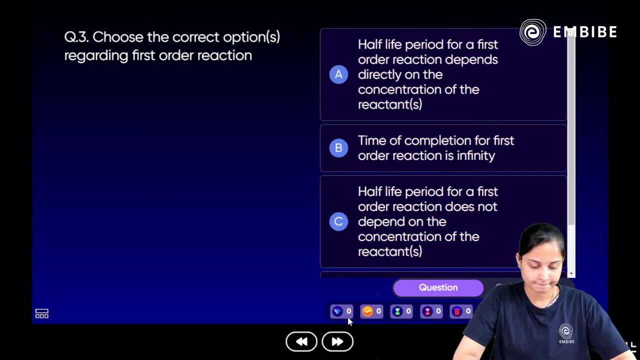 Six and three, nine. Okay, One, two, three, four, five, six, seven, eight, nine, 10,, 11,, 12,, 13,, 14,, 15,, 16,, 17,, 18,, 19,. 20,, 21,, 22,, 23,, 24,, 25,, 26,, 27,, 28,, 29,, 30,, 31,, 32,, 33,, 34,, 35,, 36,, 37,, 38,, 38,, 39,. 40,, 41,, 42,, 43,, 44,, 45,, 46,, 47,, 48,, 49,, 50,, 51,, 52,, 52,, 53,, 54,, 55,, 56,, 57,. 56,, 57,, 58,, 59,, 51,, 52,, 53,, 56,, 57,, 58,, 59,, 51,, 52,, 53,, 56,, 57,, 56,, 57,. 59,, 52,, 53,, 59,, 52,, 53,, 55,, 55,, 53,, 56,, 56,, 57,, 55,, 58,, 59,, 58,, 59,, 59,, 56,, 56,, 58,, 59,, 59,, 50,, 51,, 52,, 53,, 53,, 56,. 59,, 55,, 53,, 57,, 58,, 52,, 53,, 55,, 56,, 57,, 58,, 52,, 53,, 59,, 54,, 55,, 56,, 58,, 59,, 63,, 59,, 60,, 60,, 70,. 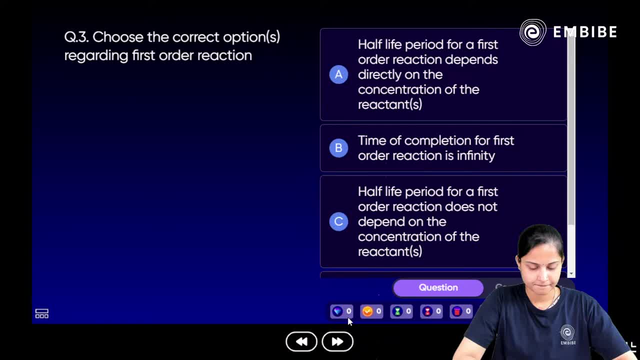 71,, 72,, 72,, 63,, 74,, 75,, 76, 78,idi row d: Nine: Two, One, Six, Three, Four. Thank you, Thank you. You must have seen it and while seeing it, you must have made it false. 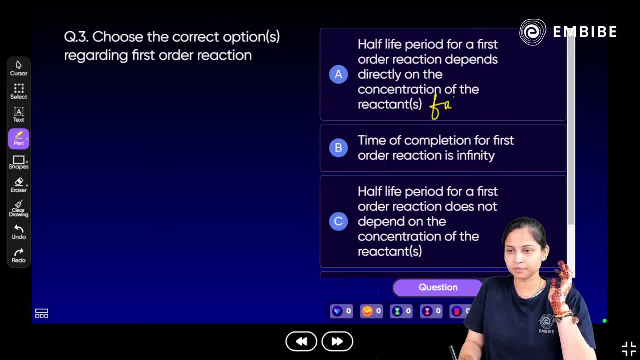 This is a false statement. I will tell you now. Now, the time of completion for first order reaction is infinity. Yes, that is absolutely true. I will actually prove it. Half life period for a first order reaction does not depend on the concentrations of the reactant. 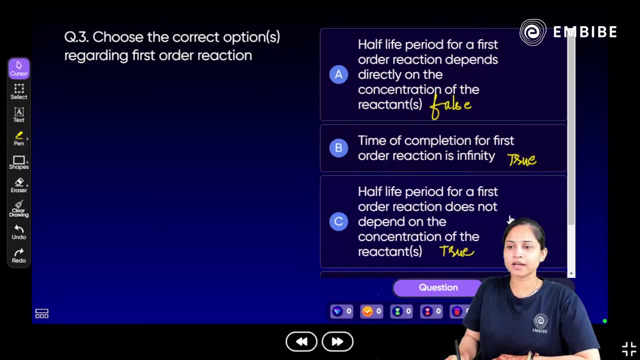 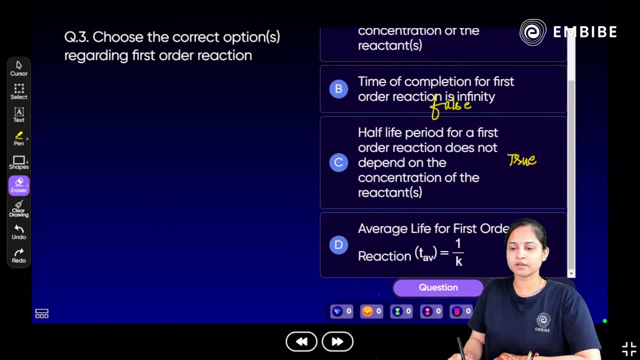 This is absolutely correct. Let's move on to the last statement. In the last statement, it is said that the average life of the first reaction for the first order reaction is 1 by k. Yes, average life is also our true statement. 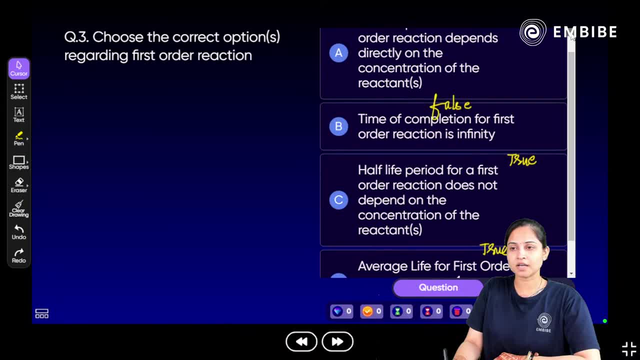 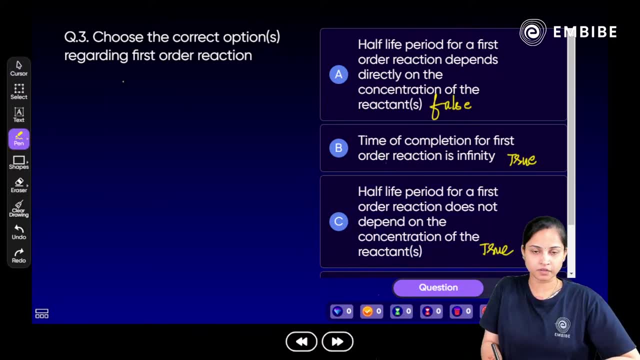 So our first three statements, no last three, I mean to say the very first statement is false and the last, b, c, d, these are the true statements. Okay, let me actually prove it one by one. We know that. 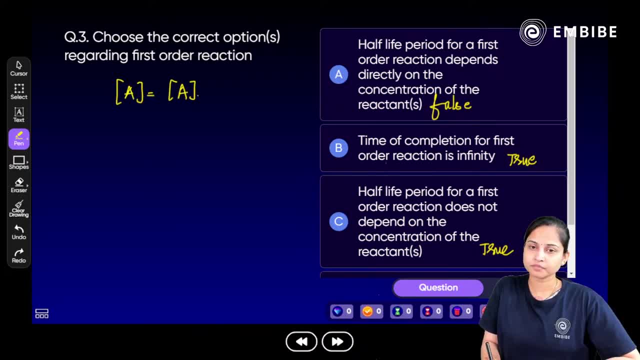 a is equal to a0. e raised to power minus kt, Exponential form. I am telling you: a0 is the initial concentration, a is the concentration at time t. This is the concentration at time t. Concentration at time t: Clear. 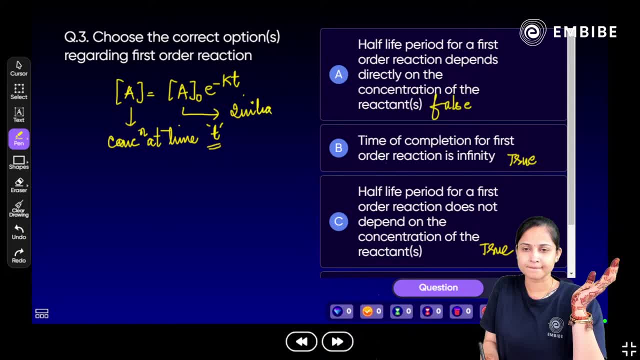 And this a0 is the initial concentration. Okay Now, if I say t is equal to t half and a is equal to a0 by 2. So if I just substitute the values, so it is basically a0 by 2.. 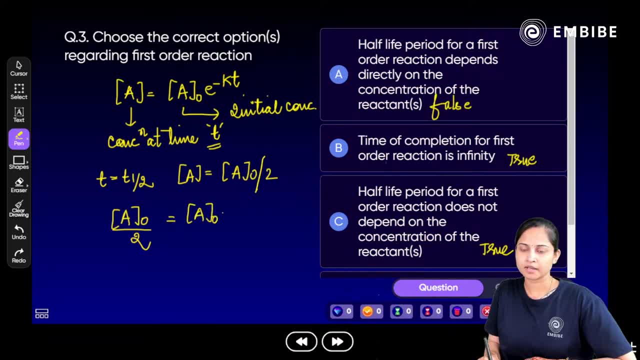 Which is equal to a0 e raised to power minus k t half. Hmm, Understood, When we solve this further, what we are going to get. that t half is equal to ln 2 by k, So half life for first order. 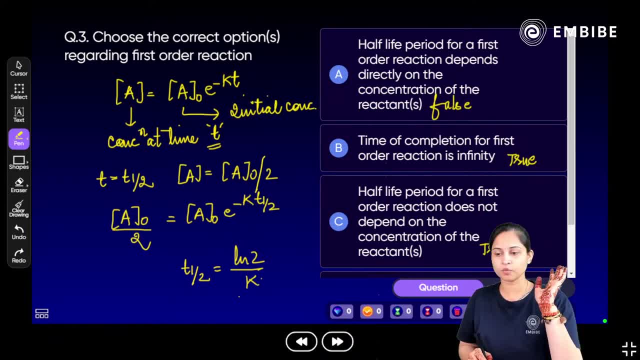 does not depend on the concentrations of the reactant, And this I have proved to you. Average life for the first order: T average for first order is equal to 1 by k. Now the time of completion of the reaction. if I just talk about. 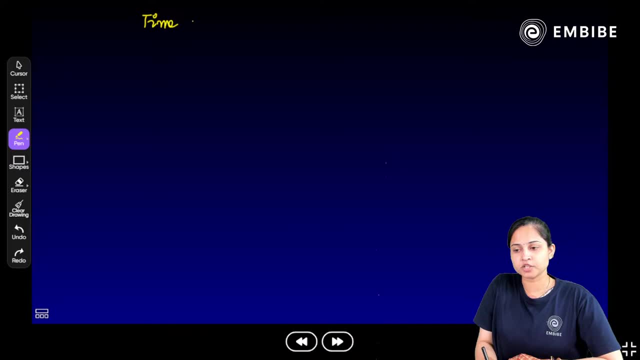 Here you will see if I just talk about the time of completion. Time of completion of reaction. Okay, So we know that a is equal to a0, e raised to power minus k, t, So at completion reactant concentration will be 0.. 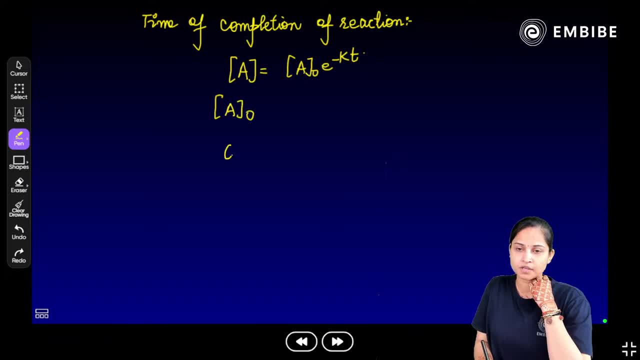 At completion, the concentration of the reactant will be 0.. So 0 is equal to what will be the concentration of the reactant. I am saying time of completion of the reaction. Okay, So at completion, the concentration of reactant will be 0.. 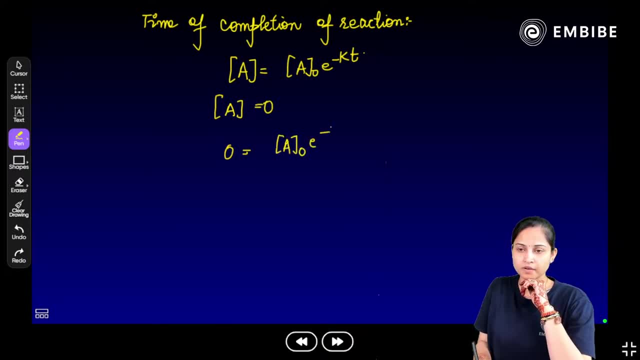 So 0 is equal to a0. a raised to power minus k, t half, If ba is important than to power minus KT. and e raised to power minus KT is equals to zero, which means T is equals to infinity. these equals to infinity, yes, so, homily, a proof, cardia. 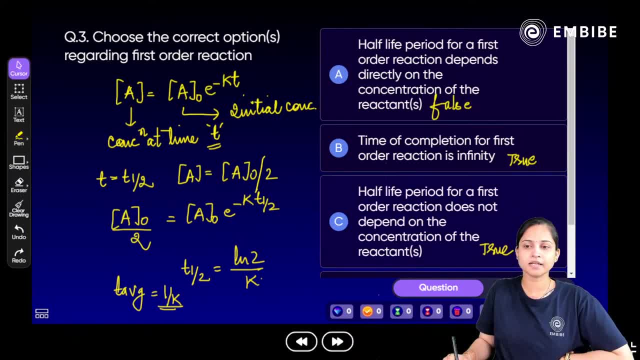 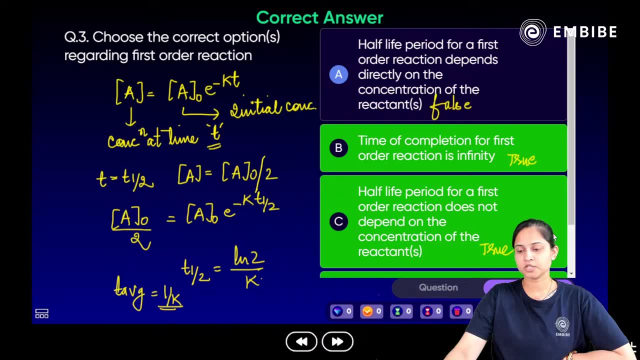 absolutely right. so, in a way, yaha per, BC and D are the right answer to the question. BC and D are the right answer to the question. basically, Hanji, shall we move ahead? our gator of prasad, kareham chalo, next question. pay him. Nick Arlene, six question of it up, let's move. and 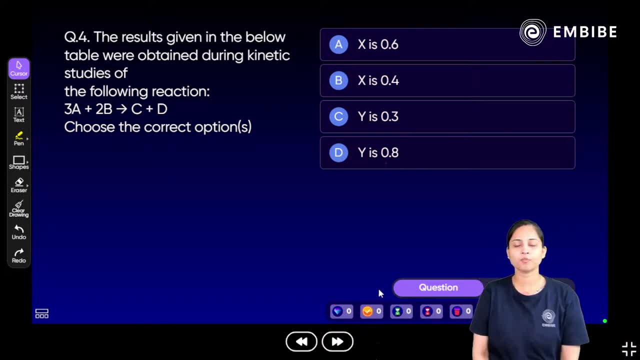 talk about this question. the results given in the below table were obtained during kinetic studies of the following reaction. you need to choose the correct option. I'll let you show the table also, but a squishing was kept cutting because table I'm a provided na here you. 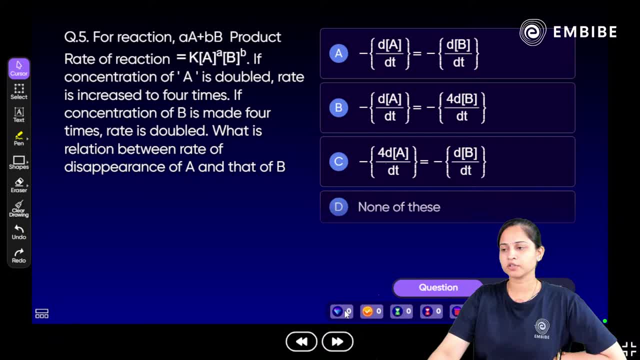 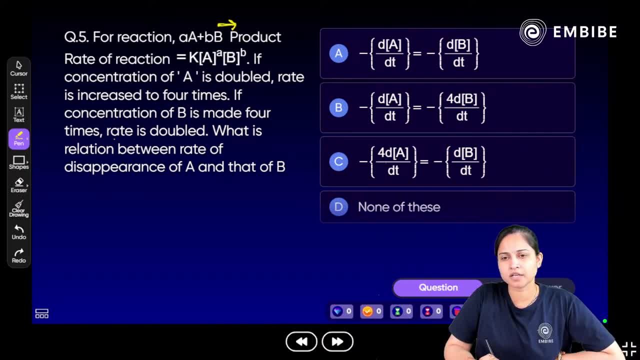 you can answer it, yeah. so the next question is in front of you. for a reaction a Barat e plus b of B. that is going to give us the product a of a plus B of d gives us the product rate of reaction is equals to k. is to PW. dear is to Politicallyback. that is going to give us the product a of p plus Bof Bey gives us the product rate of reaction is equal to case to power. a was tofour be. if concentration of a is the deliberated rate is increased to 4 times. if concentration a is doubled, rate is increased four times. if concentration appears is doubled, rate is increased to four times. if concentration is increase by two times. if concentration of Asia increased to four times. if concentration is increased to artificial disanci. 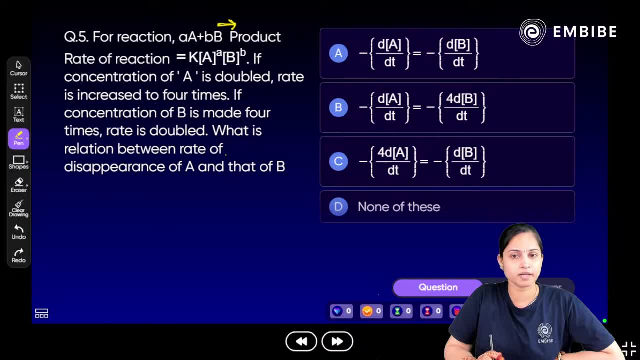 is doubled, rate is increased to four times. if concentration of B is made four times, rate is doubled. what is the relationship between rate of disappearance of A and that of B? This type of question I asked you yesterday. I am giving you two minutes time You solve this question and tell me. 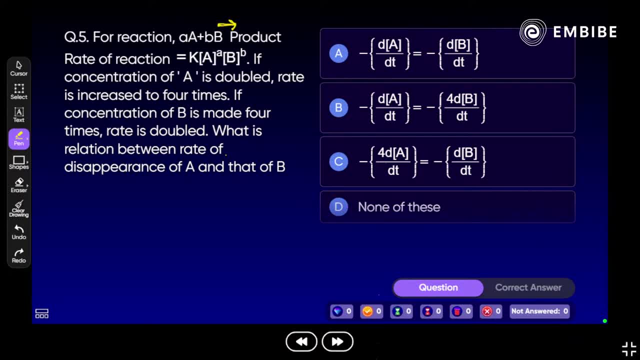 I am just watching you guys. Just let me know the right answer to the question: you, you, you, you, you, Thank you, Thank you. Okay, Let's move ahead and talk about this particular question. We have been told that if concentration A is double, rate is increased to 4 times. 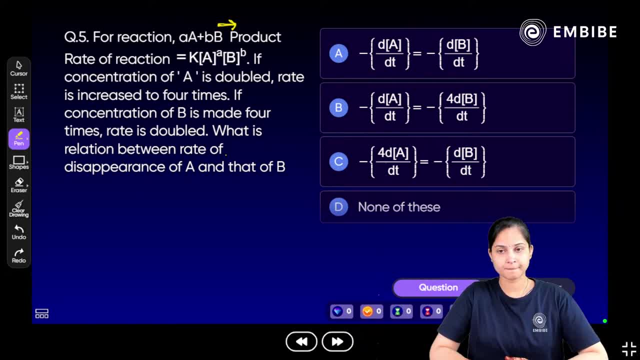 If concentration of B is made 4 times, rate is doubled. Okay, What is the relationship between rate of disappearance of A and that of B? basically, So, people here, I would like to tell you that here you will see one thing: what I literally want to talk about the same. 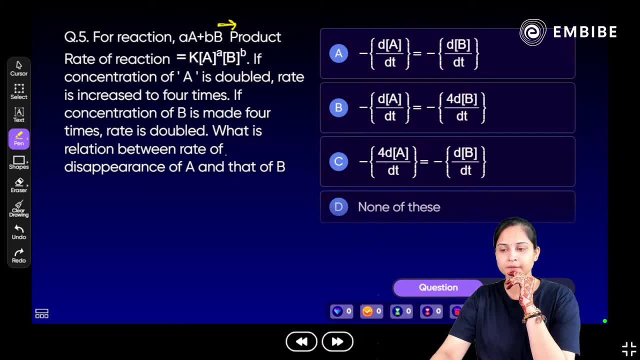 So just give me a second to go with this particular thing, Okay. So here I would like to tell you that, for this particular given reaction, what will be our rate Rate is equal to K, A of A and it is B of B. 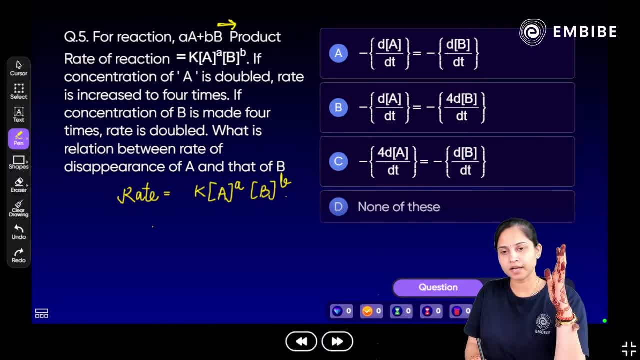 Yes. So let us consider rate of reaction B, R On doubling concentration of A, on doubling the concentration of A. so our concentration of A has become twice of A and rate of reaction R has become 4 times of R. Yes or no? 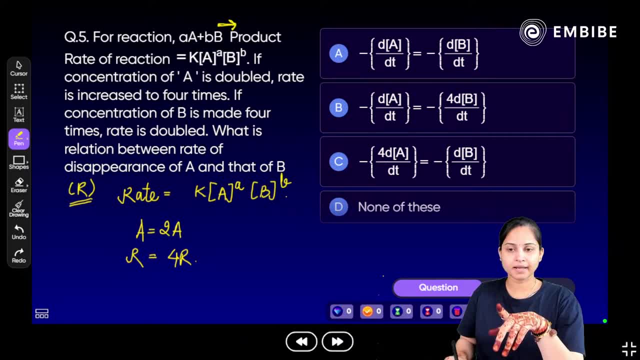 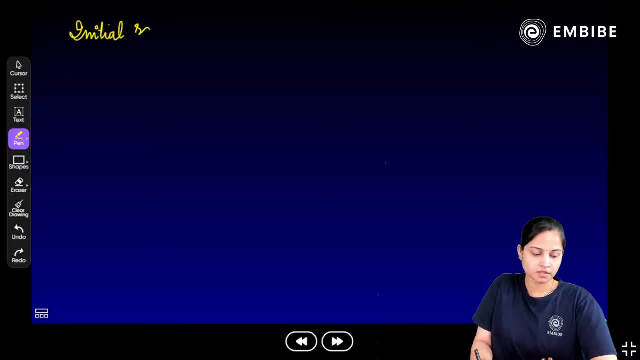 Yes, So what we actually talk about? before that, I would like to teach you one more thing: the initial rate method. Do you know initial rate method, Initial rate method. Okay, So just say R is equal to K, A raise to power P, B raise to power Q and C raise to power R. 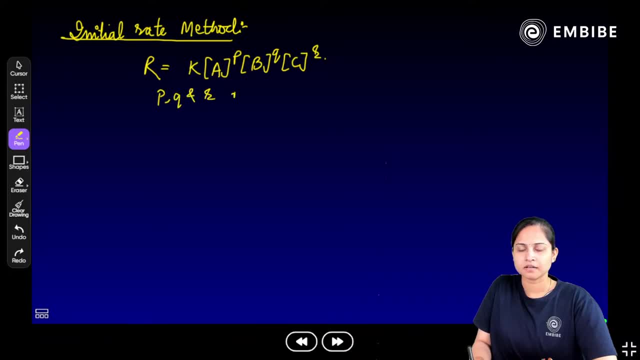 So P, Q and R are order of reactions. Are order of reaction with respect to A and B. Okay, P, Q and R are what? The order of reaction with respect to A and B. This is B. This is B. 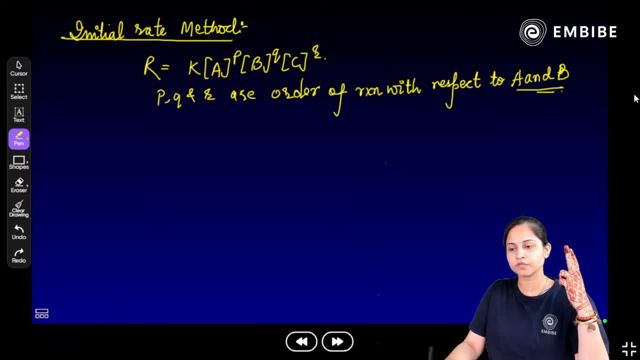 Okay. So when two different initial concentrations of A are there, Okay. When two different initial concentrations, Okay. When two different initial concentrations of A are there, That means it's A naught 1 and A naught 2 are taken. 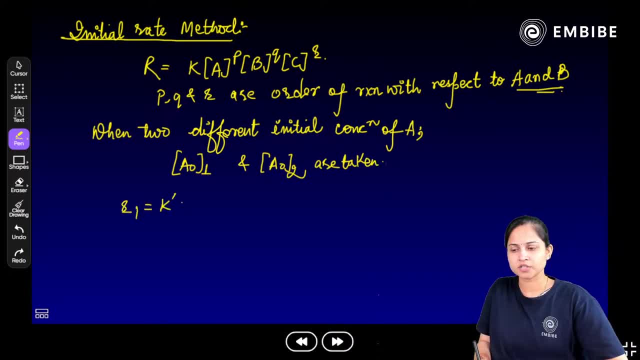 So R1 will be K dash A naught 1- raise to power P, and R2 will be K dash A naught 2- raise to power P. Okay, Yes, So in this case it will be R1 by R2, that is equals to A naught 1 and this is A naught 2.. 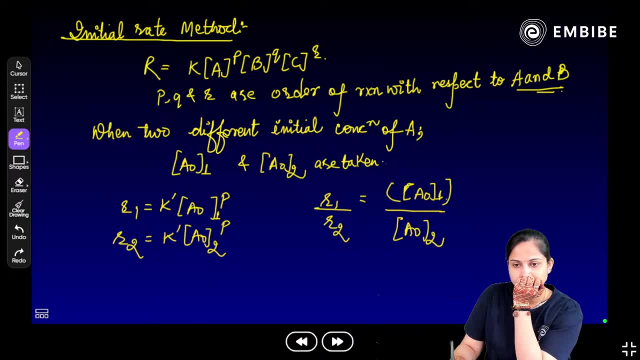 Tell me, tell me, Okay, Yeah, people tell me. And I would like to tell you one thing here: Okay, This whole is raised to power P, So what we need to calculate is P. From this relation, P can be calculated. 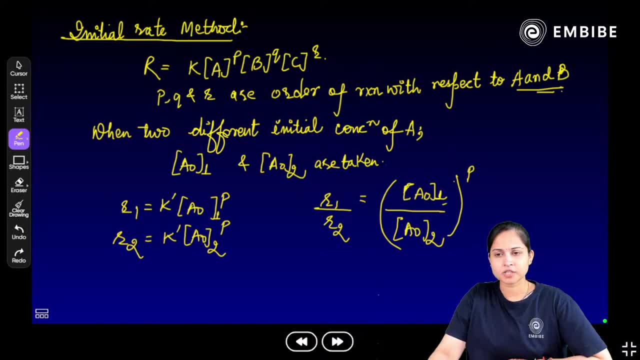 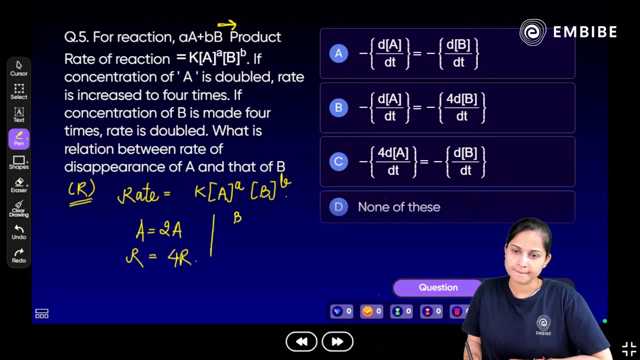 Okay, So it is from P, so R1 from R2. we have found the solution by Hawking diode. So if we, if we have completed charging, then we subtract through P so we get Alright. If to find the solution of the equation in the initial concentration of A, we have given. 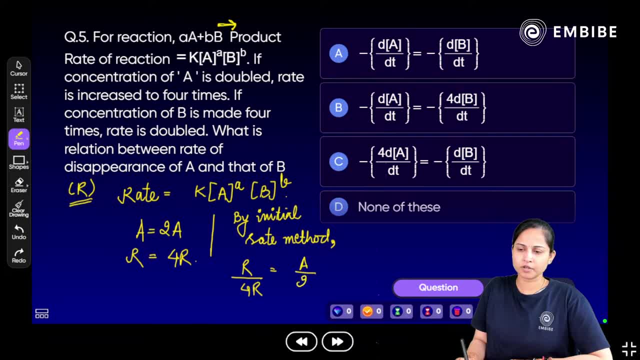 r, which is equals to a upon twice of a raised to power a. so r cancels out with r, so it becomes 1 upon 4, is equals to 1 upon 2 raised to power a, so here it will be 1 upon 2, whole 2 equals. 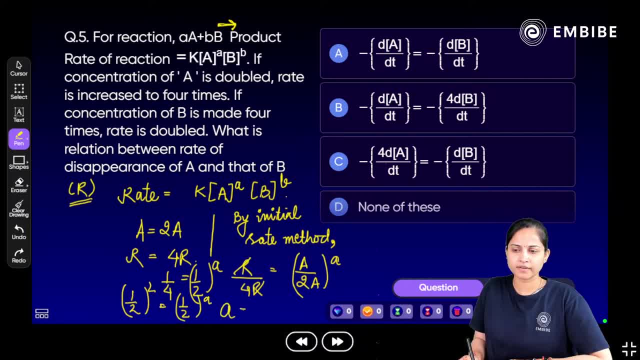 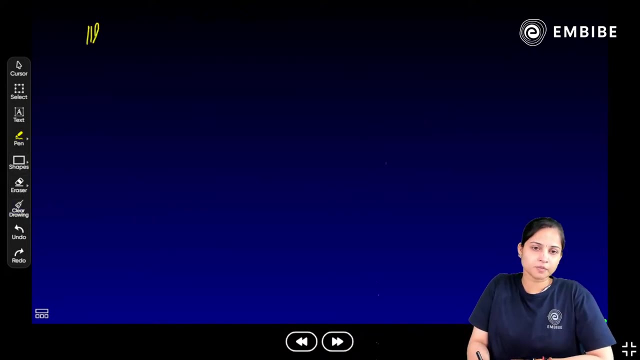 to 1 upon 2 a. so in a way our value of a has come to be 2. we have done here in respect to that, when we came to know that if concentration of a is doubled, if concentration of a is doubled, rate is increased to 4 times. ok, is it clear now? similarly, if I talk when b. similarly, 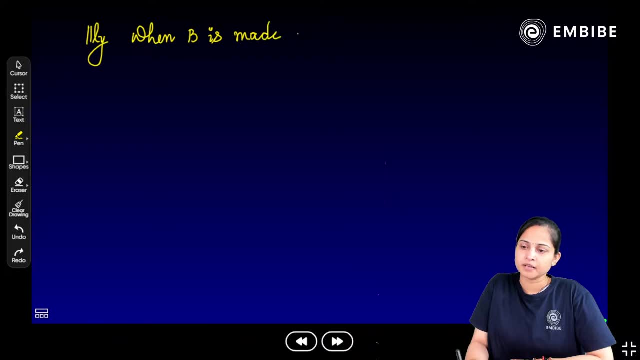 when b is made to, when b is made to 4 times, the rate of reaction is doubled. when b is made to the rate of reaction, the rate of reaction is doubled. so here see r upon twice of r, that is equals to b upon 4 times of b raised to power b, so it will be 1 by 2 equals. 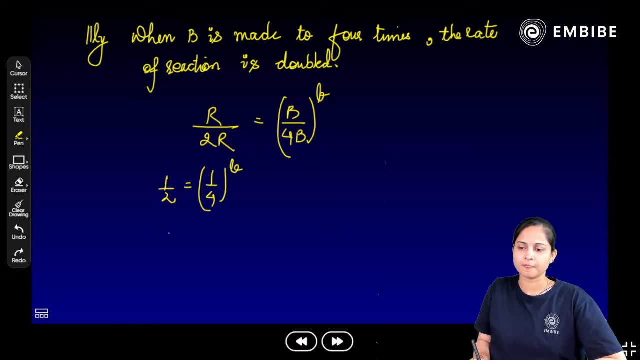 to 1 by 4 raised to power b. yes or no, people tell me. so now, what will be the value of b here? what will be b? b will not be half. it is half raised to power. half equals to 1 by 4 raised to power b. so b is equals to half. 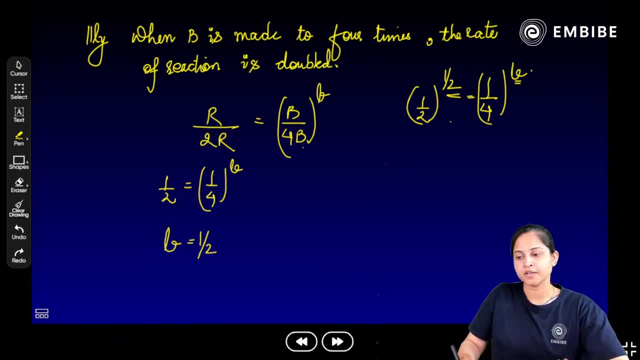 ok, so what will be the value of b? here it is half. so rate of reaction, rate of reaction, r o r, what is it? it is k, a raised to power 2 and b raised to power half. so what we can say it is twice of a plus half of b, giving us the product. yes, tell me. this question is: 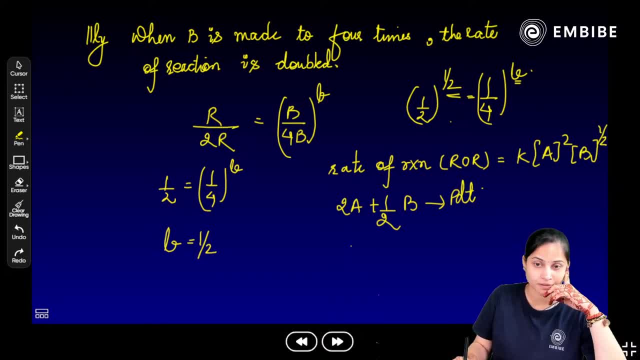 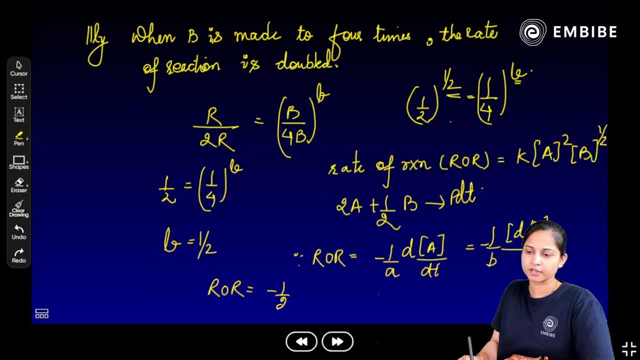 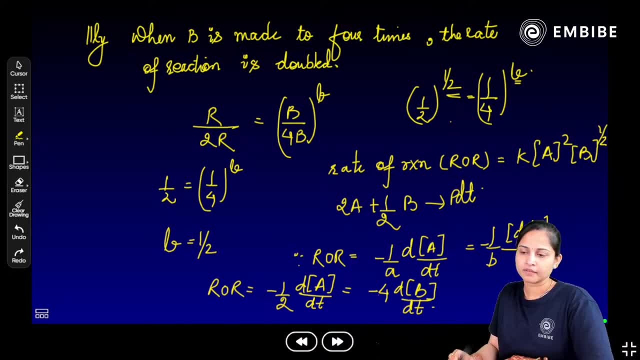 Tell me, are we doing this right or not? We made a mistake One minute. I only made a mistake Directly. 4 will not come here. It will be how much Minus 2.. Now, when this 2 will go here? 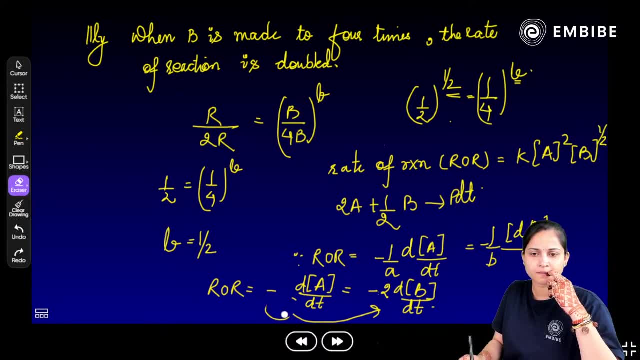 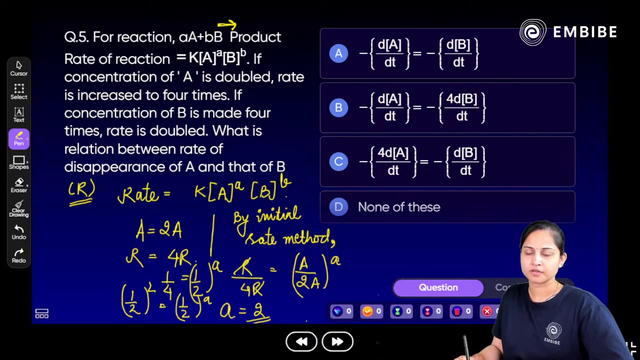 so what can I write it over here? Minus 4.. So minus dA by dt is equal to minus 4 dB by dt. Minus dA by dt is equal to minus 4 dB by dt. According to that, option B is our correct answer. 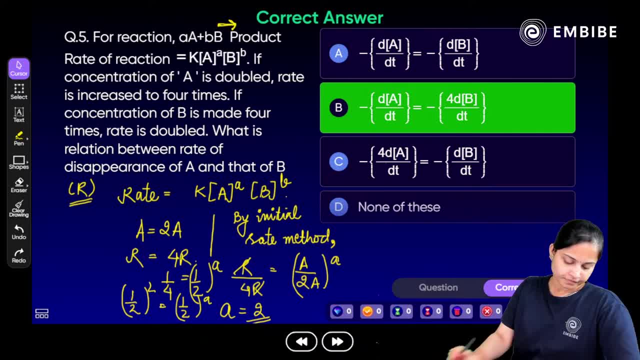 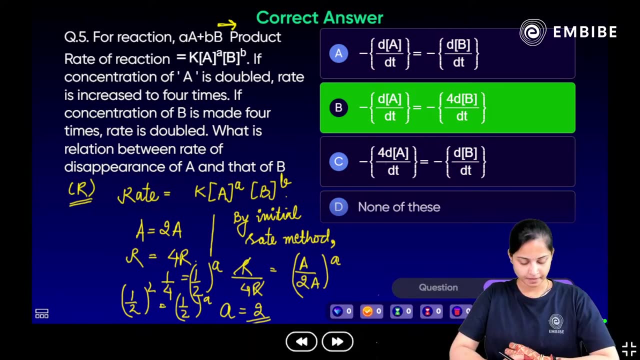 Because this is the timing of NEET's channel. Because this is the timing of NEET's channel pair. NEET's session starts from 11 to 12.15.. That is the main reason Understood Aditya Babu. 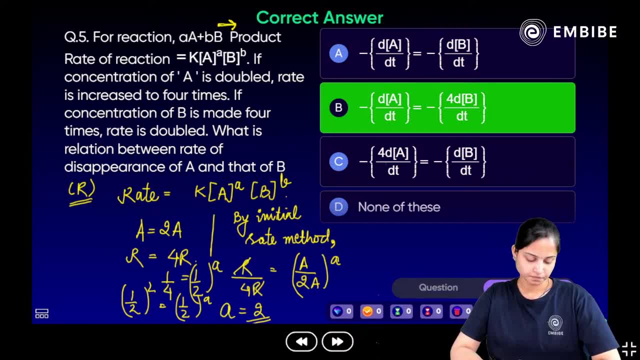 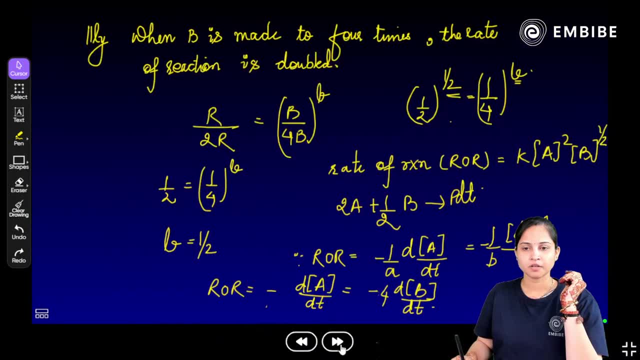 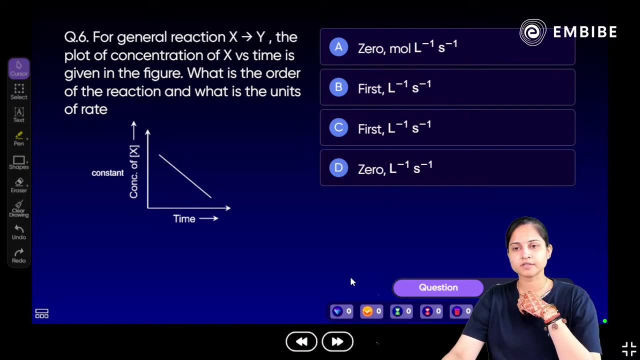 Yes, we understood. Yes, it was thePLOTZ. That was the main reason. Yes, it was the main reason. Next question. Let's go on to the next question. See the question carefully, understand and tell. For the journal reaction x to y, the plot of concentration of x versus time is given in the figure. 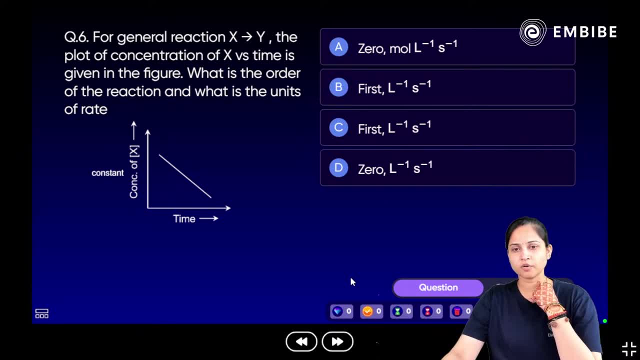 What is the order of reaction And what is the unit of rate? This is the graph of concentration versus time. This is a graph of concentration and time. The average is 0.. And this is the answer? Yes, is it right? 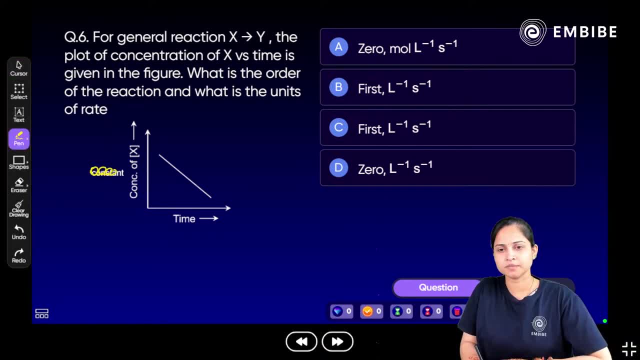 what is the order of the reaction? what is the unit of rate constant? what is the order of the reaction? what is the unit of rate constant for zero order? if we calculate this much for zero order, our rate law equation is basically: a0 minus at is equal to kt. 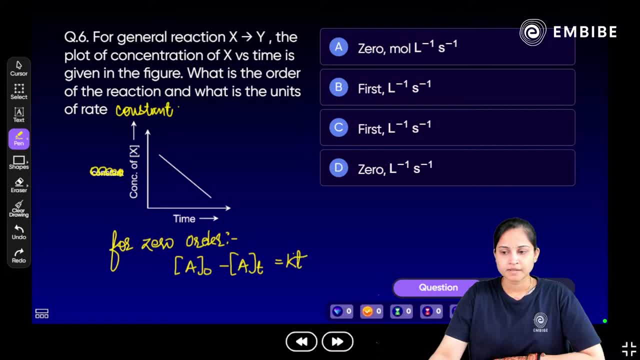 we solved this also in the back, yes or no? yes, it was so. from here we know: at is equal to a0 minus kt, and this is in the form of y equals to m, and this is in the form of y equals to m, and this is in the form of y equals to m, x form. so the plot between 80. 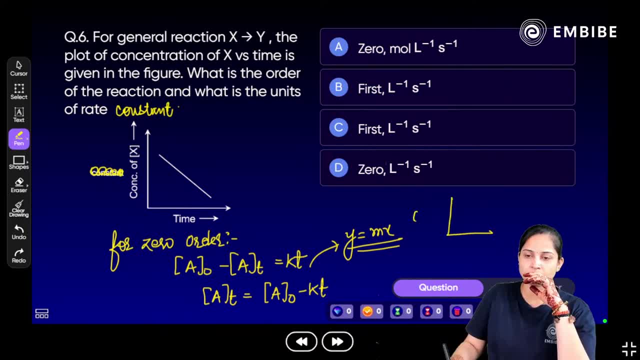 x form. so the plot between 80: x form. so the plot between 80. concentration versus time T. yeah, they concentration versus time T. yeah, they concentration versus time T. yeah, they cook concentration. have a repass me cook concentration. have a repass me cook concentration, have a repass me versus time T. and it's for zero order. 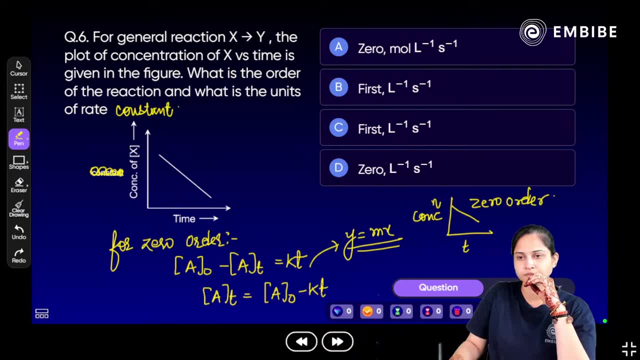 versus time T and it's for zero order versus time T and it's for zero order reaction. so you are option. a Mara say reaction, so you are option. a Mara say reaction, so you are option. a Mara say you wanna change and the unit will be. you wanna change and the unit will be. 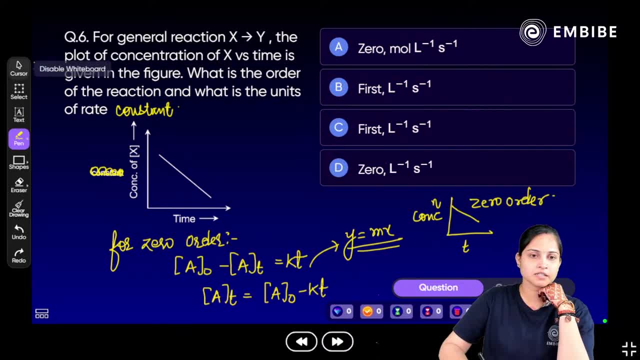 you wanna change and the unit will be moles per liter per second. you all know moles per liter per second. you all know moles per liter per second. you all know. so option is the right answer to the. so option is the right answer to the. 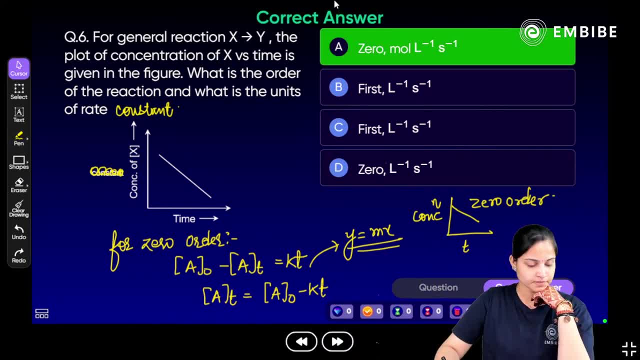 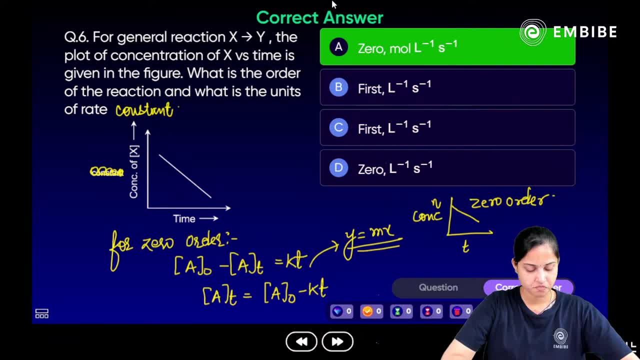 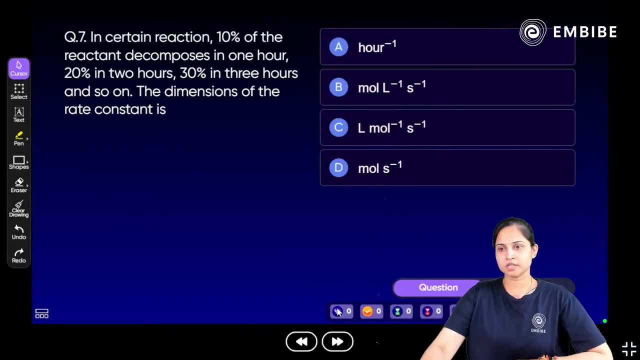 so option is the right answer to the question. so option is the right answer to the question. so let's move on to the next question. so option is the right answer to the question. so option is the right answer to the question. so answer this question. so option is the right answer to the question. so answer this question. 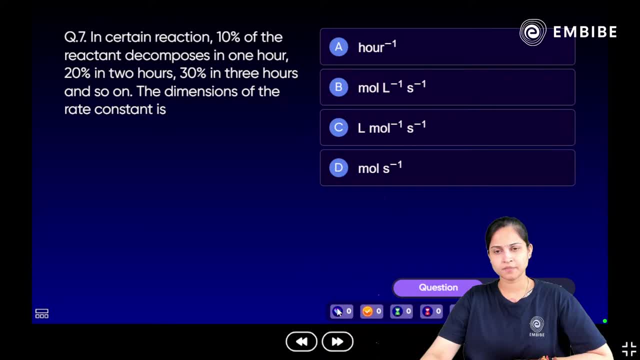 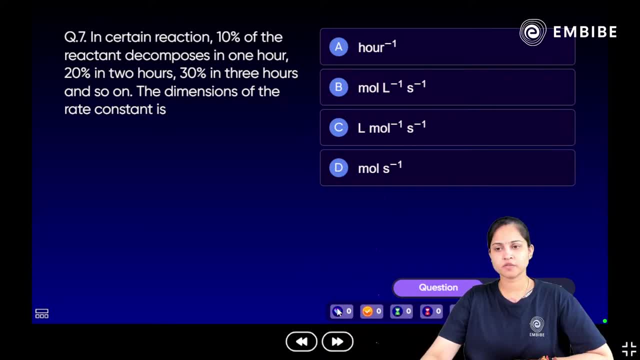 so option is the right answer to the question. so answer this question. in certain reaction, 10% of the reactant decomposes in one hour. 20% in 2 hours. 30% in 3 hours. dimensions of the rate. 20% in 2 hours. 30% in 3 hours. dimensions of the rate. 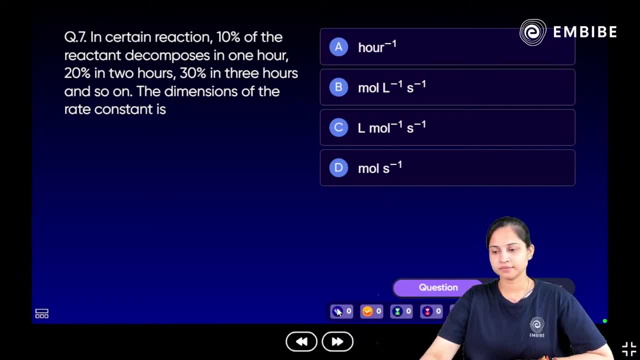 20% in 2 hours, 30% in 3 hours. dimensions of the rate: constant is constant is constant. is that's a question about? that's a question about? that's a question about? but I think I question, hmm, hmm, hmm, tell you, tell you. 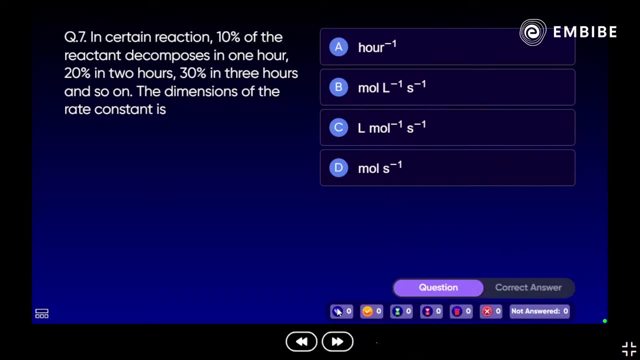 tell you I'm going to question on the screen. let me. I'm going to question on the screen. let me. I'm going to question on the screen. let me know the right answer to the question. know the right answer to the question. know the right answer to the question. waiting for your answers. 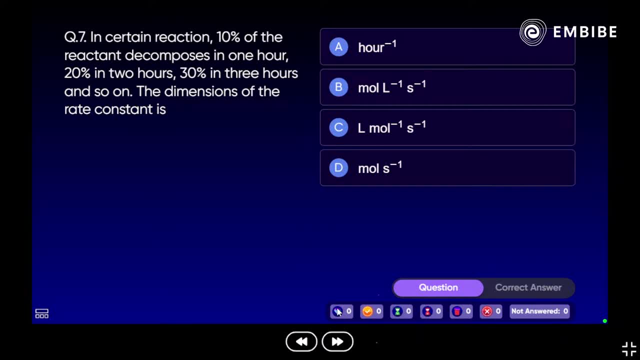 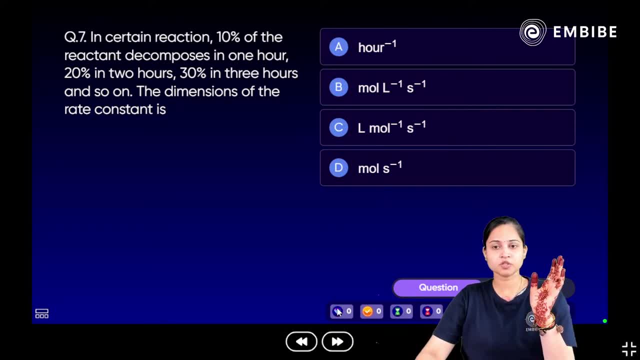 20% in 2 hour, 30% in 3 hours and so on. Dimensions of the rate constant You are asking here. See, Often we're amazed the given reaction is a zero-order reaction. Q, because I'm plotting the percent composition of a reactant. take a person. composition of the reactant left. 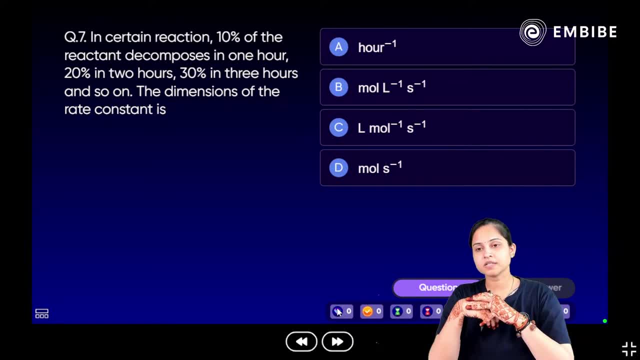 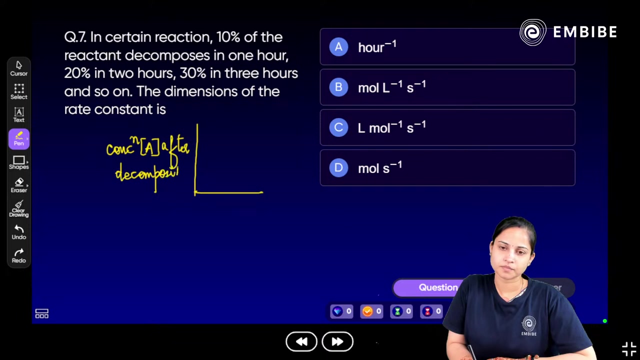 after decomposition of the reactants versus time T, we will obtain a straight line basically. so I put: which is the Nika graph Milligan. you happen mechanically, you concentration of the reactant after decomposition, after decomposition percentage, and this is time T in ours. so I put: which is a graph Milligan, so this particular given reaction. 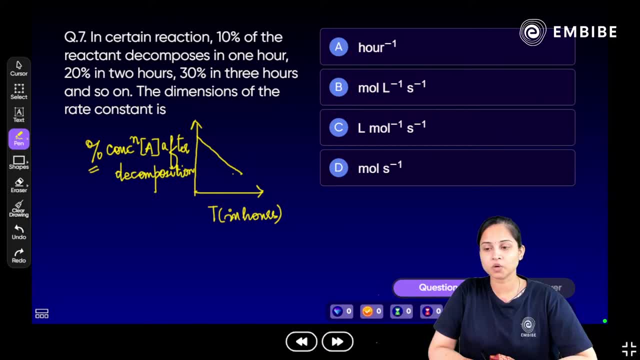 is a zero-order reaction Q because I put, which is the Nika graph Milligan, so this particular given reaction is a zero-order reaction Q because I'm plotting the percent concentration of reactant left after decomposition of reactants versus time. T will be obtaining the straight line. now for zero-order reaction: concentration versus 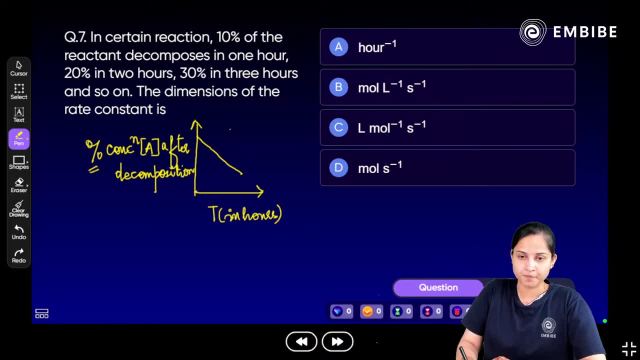 time graph is a straight line with a negative slope, straight line with negative slope. so if I just consider a zero-order reaction people, so what? to which particular extent we reaches? we reach by 80 z equals 2. a naught minus katie ate is equals to pinky knot minus Katie, basically. so it is in which particular. fall IZ equals two minus M, a, z minus K, suppose this is real. so if I take this one, this is real. so this is real. so if I take this one, this is real. so this is real. so if I take this one, this is real. so if I take this one, the short term is ok for them. how many of you? 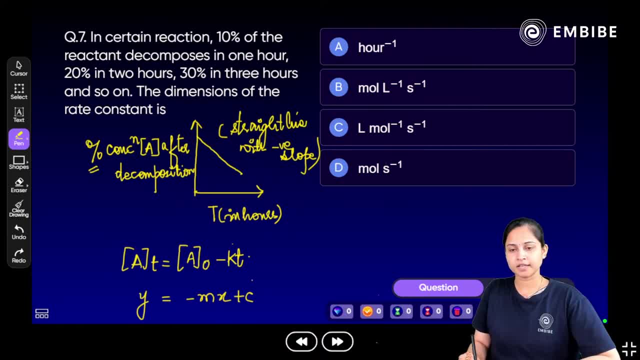 the short term is ok for them. how many of you? they are equal to each other. so if I take this long term, it will be out according to mx plus c wale form mein hai. Hence the order of the given reaction is 0.. Rate kya hai. 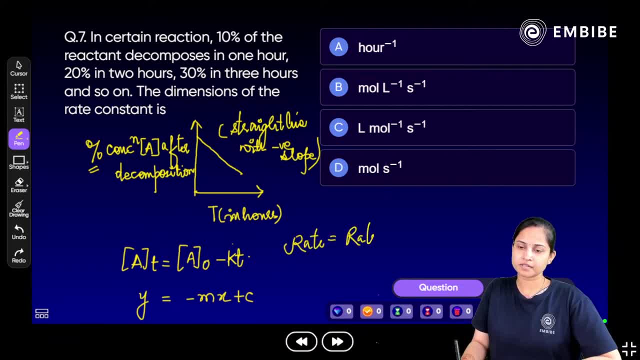 Rate is equals to rate constant. Rate is equals to rate constant. That is equals to dx by dt. So 0 order ka hamara unit. kya hota hai? Moles per liter per second? inverse. Option B is the right answer to the question. Yeah, people, let's move ahead and talk about the 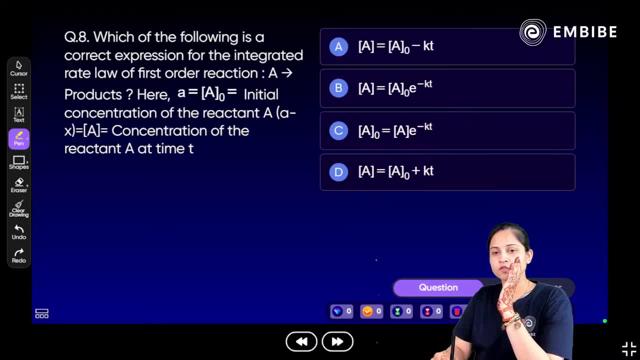 next question. now, Here we are on to the next question. Which of the following is a correct expression for the integrated rate law of first order reaction A to product hai? Here, A is equals to A0,. the initial concentrations of the reactant: A minus x is equals to A. 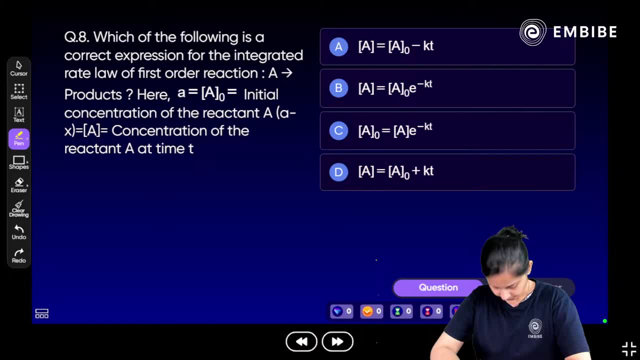 concentrations of the reactant A at time t Batayenge aap mujhe yaar par. Kaise yaar batayenge The integrated? Yeh toh waise solve karne ki zarurat nahi hai. Dekhte hi aapne. 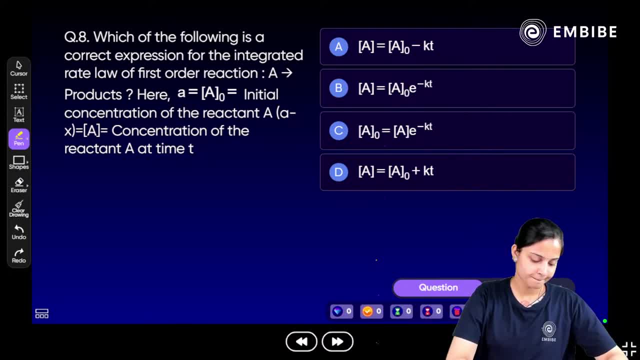 yaar bata diya hoga. Tell me the right answer Friday. Nareed mokhi aapman piya hain, Bhwa Kaise hai? Kaise hai aapman piya hain Baareyo mokhi hai. 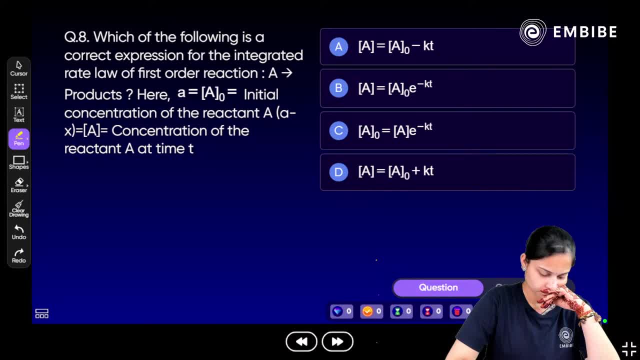 Baareyo yi hai, Baareyo mokhi hai. Kaise hai Baareyo yi hai, Baareyo mokhi hai. How many half-lives do you have? How many half-lives should be elapsed for first-order reaction so that the reaction is 95% completed? 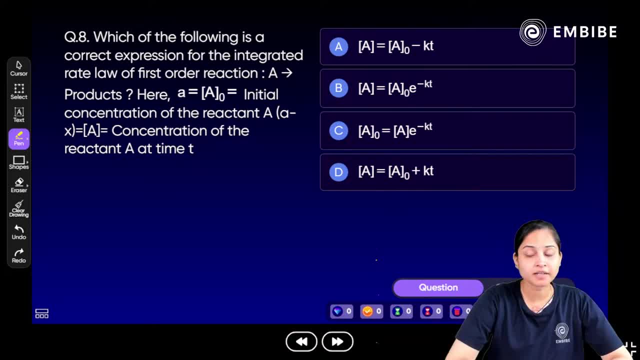 How many half-lives must have been elapsed just so that the reaction is 95% completed for first-order reaction? Are you asking this? Are you asking this In order to get the 95% reaction to get completed? I will tell you about this particular question. 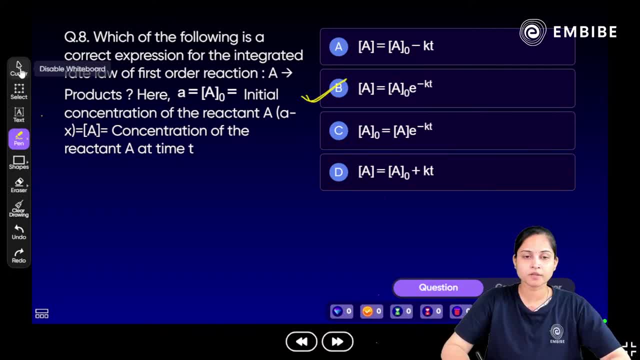 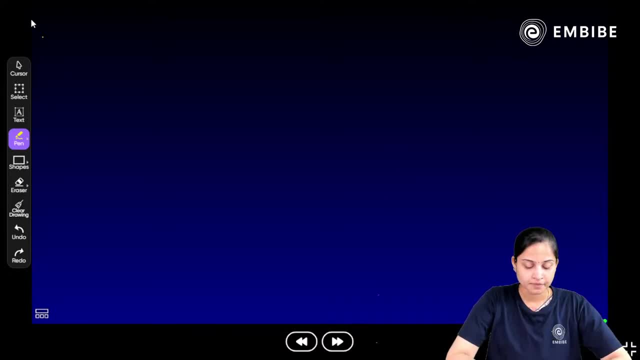 So its answer is option number B. A is equal to A0, E raised to power minus KT. Now what you asked me? you asked me how many half-lives should have been elapsed for first-order reaction. How many half-lives should have been elapsed for first-order reaction so that the reaction is at least 95% completed? 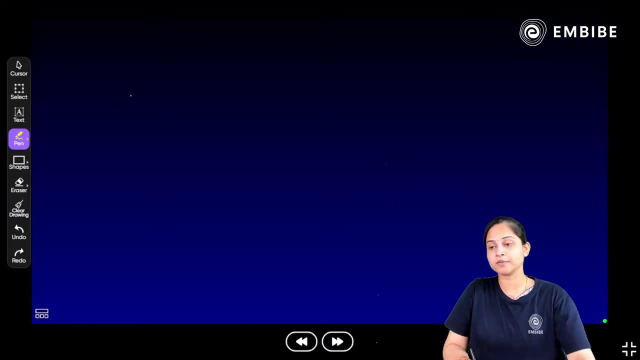 So, dear one, 95% reaction is completed. So you see, here from 100, when we go to 50,, so here T is half, so here 0% is completed, but here 50% of the reaction is completed. 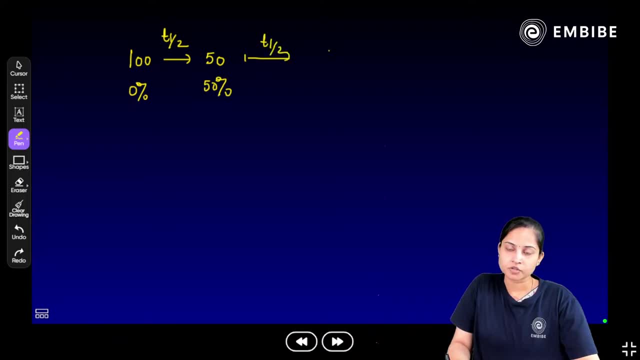 Then we will go forward. then T half will come. so here 25.. So here 0,, here 50, and here 25.. So here 75% of the reaction is completed. Now, if we do T half of this, then we will be getting 12.5.. 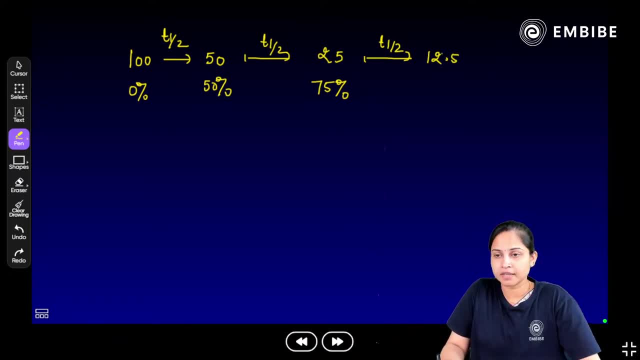 Yes or no. So now you see here what we have done for this. we have done 12.5, dear one Yes or no. T half of 25 is 12.5.. So here how much percent of the reaction is completed. 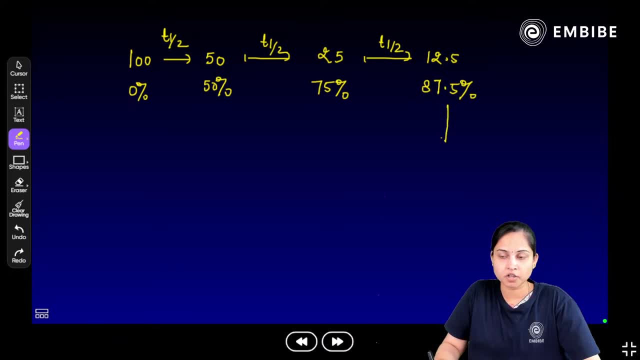 Here, 87.5% of the reaction is completed. Further on, when you do T half of this again, so it will be 6.25.. So here, 87.5% of the reaction is completed. Here, 87.5% of the reaction is completed. 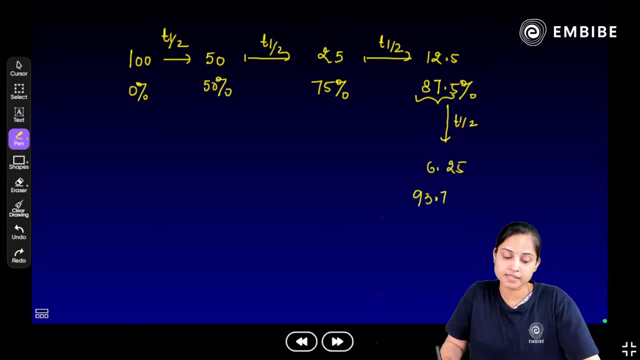 Here the reaction completed will be 93.75% of the reaction is completed. Further, if you do T half of this, so you will get 3.125.. Yes, So now you see, here it is 93.75, I will add 3.125. 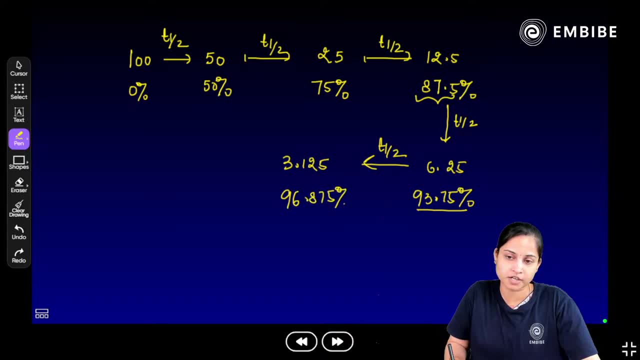 So it is 96.875% of the reaction is completed. So how many half life You are going to elapse in order to get that? the 95% of the reaction is completed when we are talking in case of first order right? 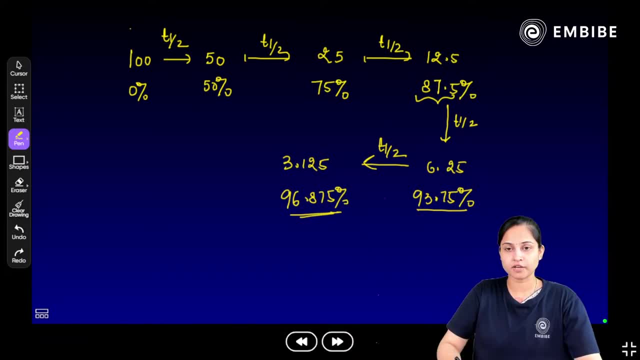 Yes, So it will be 1,, 2,, 3,, 4, 5.. It is 1,, 2,, 3,, 4 and 5.. 5 half-lives. 5 half-lives, dear one. 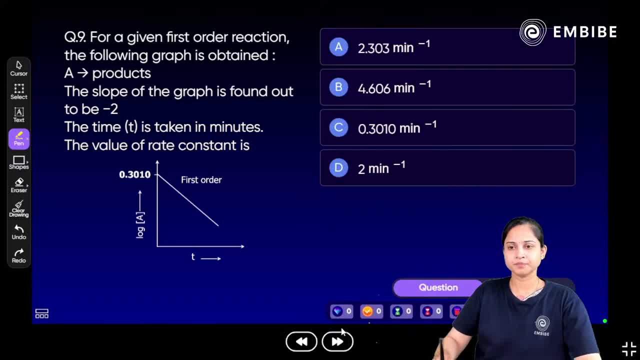 Okay, Let's move on to the next question. Hmm, Now tell me about this question. For a given first order reaction, the following graph is obtained: A2 product: The slope of the graph is found out to be minus 2.. 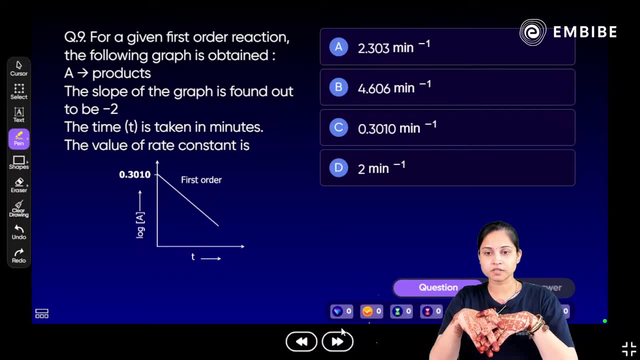 The time t is taken in minutes. The value of rate constant is. You have to tell the value of rate constant, So you have some idea of this. We know one thing here with clarity: What: That for the first order reaction, ln A0 by A is equal to kT. 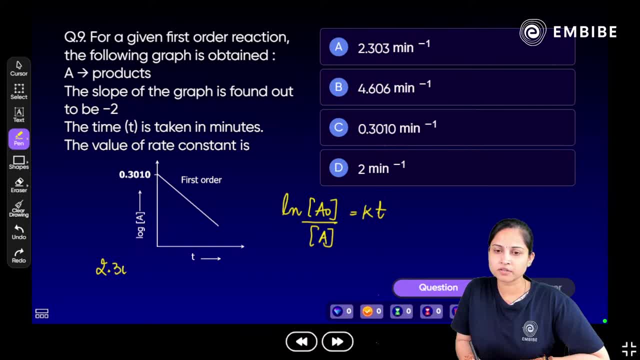 How can we write this? 2.303 by T? Yes, ln. A0 by A is equal to k. basically, Let's do it like this. This is how we do. Yes, If I want to write it in a different format, I can write it like this: 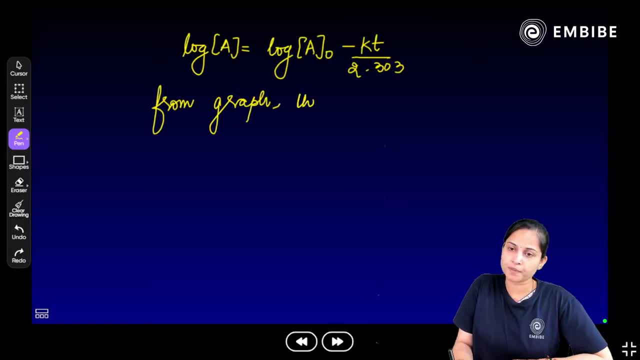 ln F. The slope is Minus k upon 2.303.. That is equals to minus 2. that has been given to us the slope. So from here, what is the value of k? 4.606 minute inverse has come. 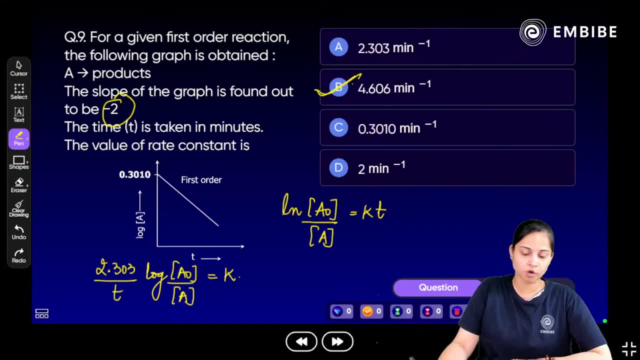 So we will be marking 4.606 minute inverse to be option. the right answer: Yes, But if you know this thing, tell me. If you understand it, then tell me that. yes, Rakhi ma'am, we have understood this. 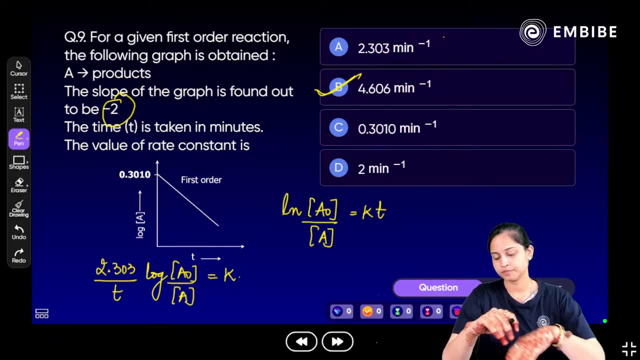 thing very well. Yes, guys, tell me. if this is absolutely into your brains, Tell me, because we have done these questions after 3, 3.6 and 3.9.. That we have done near about 12 to 13 questions till now. 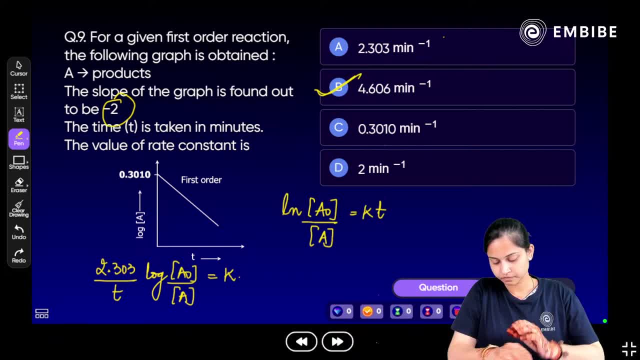 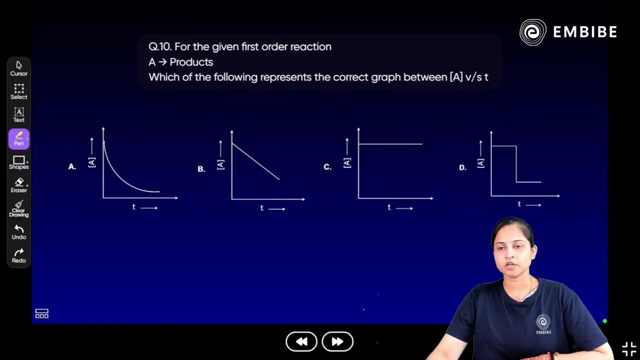 Let me know Chalye. next question: pe chalte hain. Okay, a good question in front of us For a given first order. reaction A to product. which of the following represents the correct graph between concentration A versus time t? 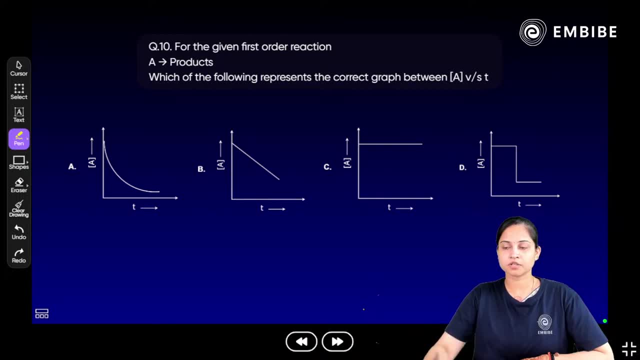 Concentration A versus time t. Okay, tell me concentration A versus time t. We know that A is equal to A naught, E raised to power minus kT Exponential graph. So according to that, your option A should be absolutely correct. 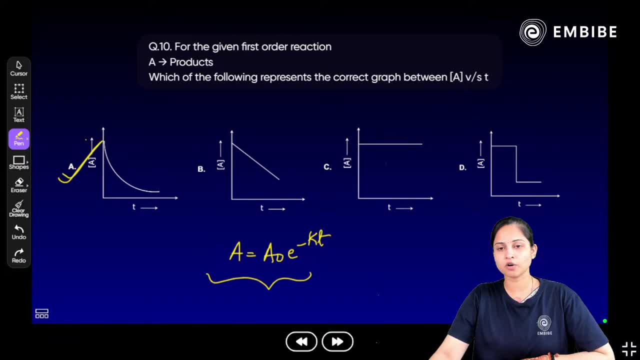 Tell me people, Yes or no? The integrated rate law of first order reaction. Integrated rate law of first order reaction ln. A naught by A is equal to kT. So from here, what will we get to know? We will get to know that A is equal to A. 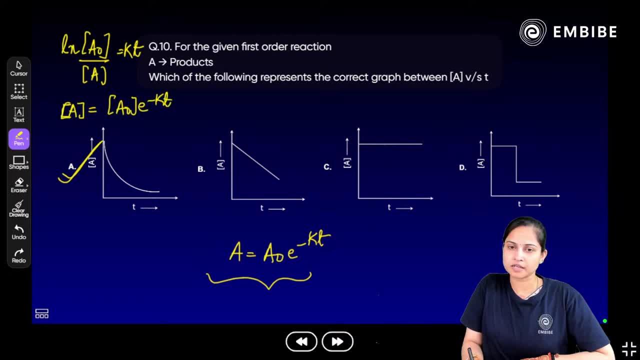 A is equal to A naught E raised to power minus kT. So from here, what we will get to know is that A raised to power minus kT- This is the two-point line- A is equal to kT, which is the world's largest mass of carbon dioxide. 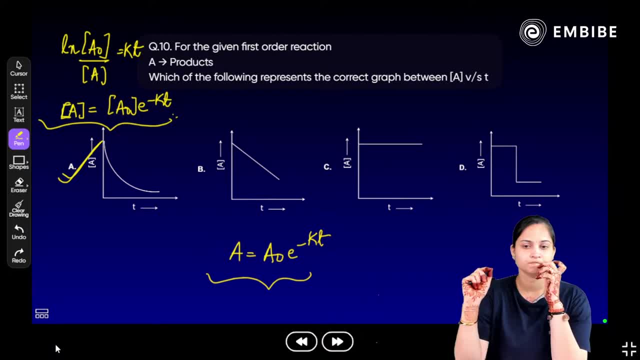 So t is equal to kT raised to power minus kT. So the two-point line is that kT is equal to kT, which is equal to kT raised to power minus kT. All right, you know what? 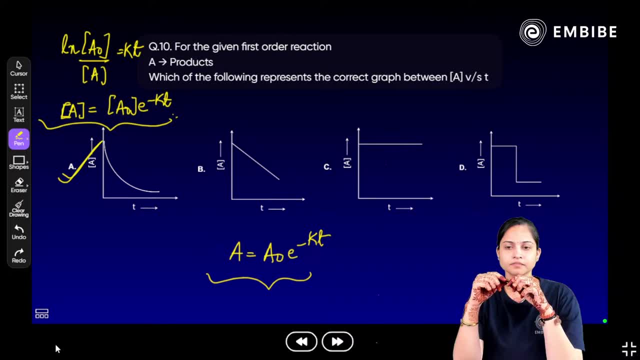 I just want to go back to the first order reaction. What we have to do is go back to the first order reaction. So in this particular example here we will get the result of our initial physics. okay, and the next question I'm giving you for the homework for the given first. 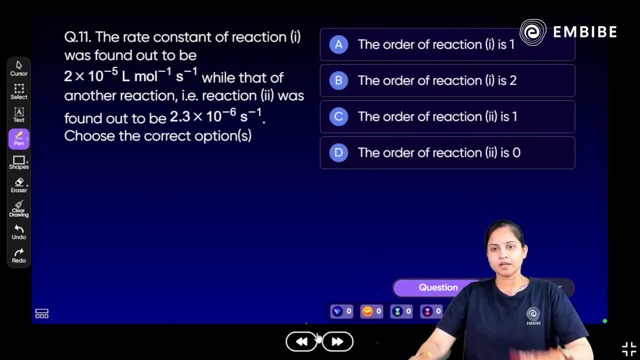 order: eat on me, Carilla, be heavy. eleventh question: the rate constant of a reaction was found out, found out to be 2 into 2 minus 5 liter mole inverse, second inverse, while that of the another reaction, 2, was found out to be this much. 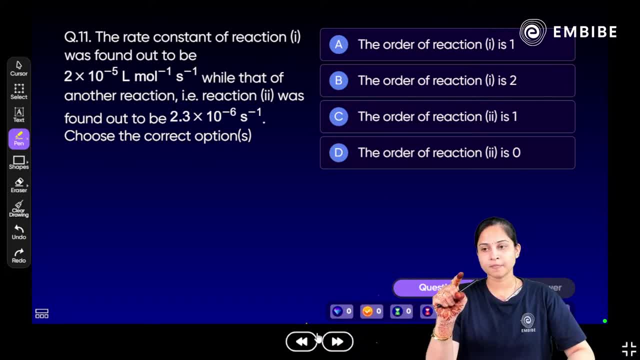 okay, they put the second Amara. hey, it's the first order. the order of reaction for second is 1. the order of reaction for the second is 1: you. the order of reaction for the second is 1. yes, okay, I quit, not a birthday yoga kejo, Hamunit of king, you can't be in a bit of a kiss.